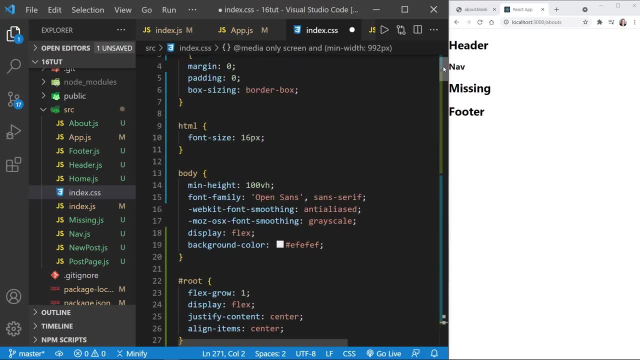 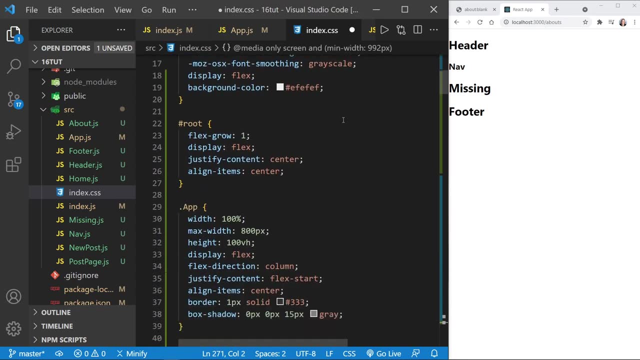 all of this CSS as well, Because I'm not going to go over all of the CSS as I want to focus on the React part of this tutorial, But the CSS will be available to you And, of course, I encourage you to experiment with CSS and style this blog. 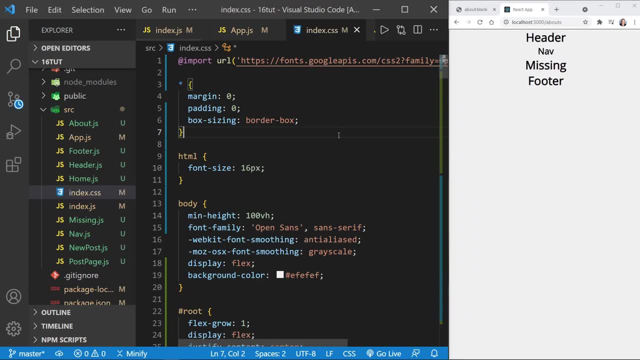 how you would like it to be. You don't have to use my styles, But I'm going to go ahead and apply that now And you can see the changes over here in Chrome have already applied somewhat And we're not seeing a whole lot. But we need to build out our components And then we'll see more of these changes as we apply. 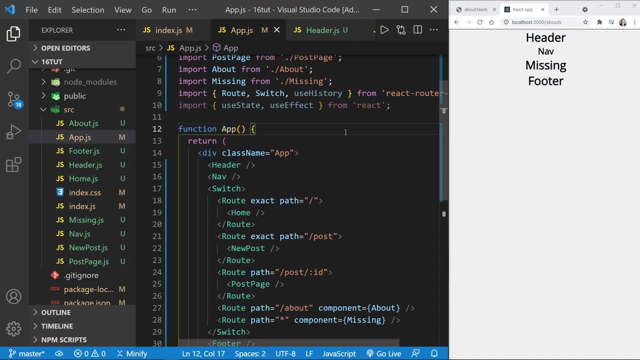 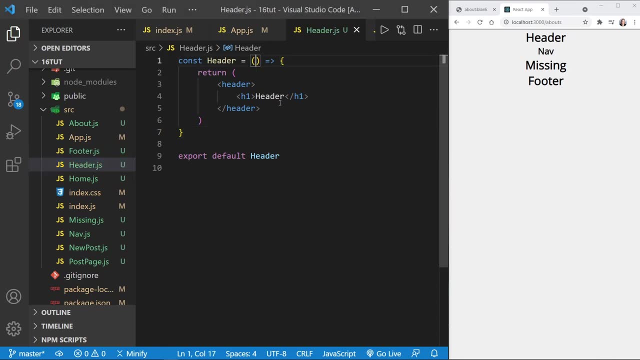 the class names that exist. So I'll close the CSS for now, And our first component is a header, So let's go to our header component. We don't have too many changes to make in the header component, But it is going to receive a title prop. 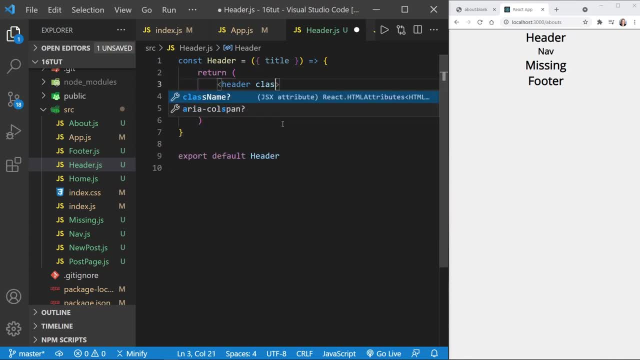 And then also the header component will have a class name attribute. This needs an extra S and a capital N. There we go, And this is going to be header as well for the class name. And then instead of saying header here in the H1, it's going to actually use the title prop to display. 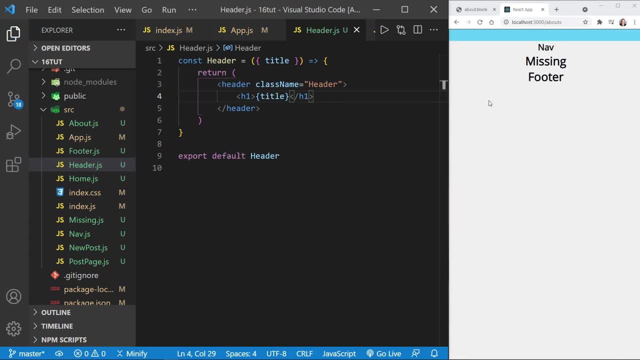 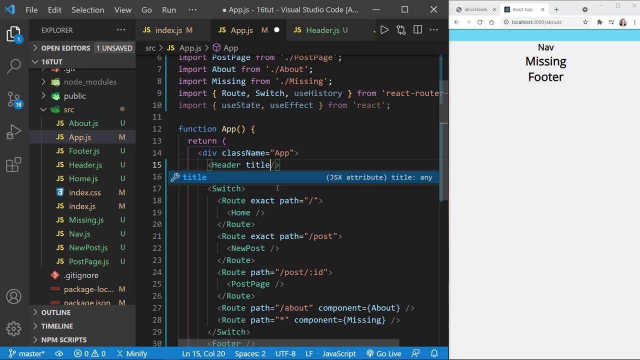 So we can save that And we might get an error Because- no, it's just blank, Because we haven't passed the title prop. Okay, So if we go back to the appjs, here in the header, we can now pass the title prop And we'll just say reactjs- blog And we'll save. 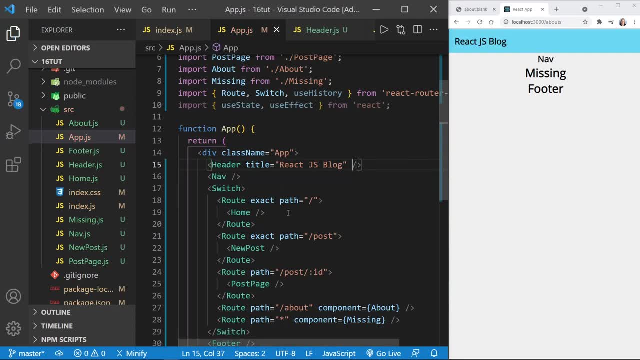 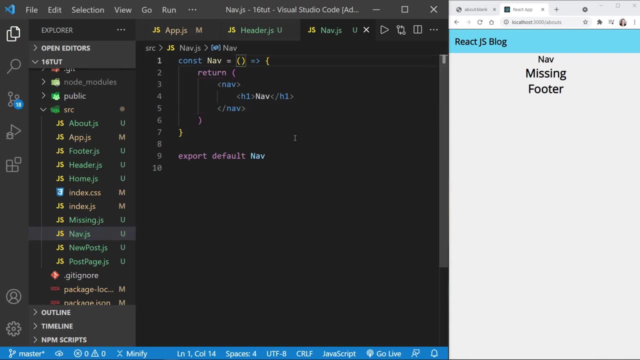 And we should now see that in the top, And we do So. that is our header for now. Let's move on to the navjs, which is the next component, And we've already got the nav element. Now nav is going to receive search and set search. 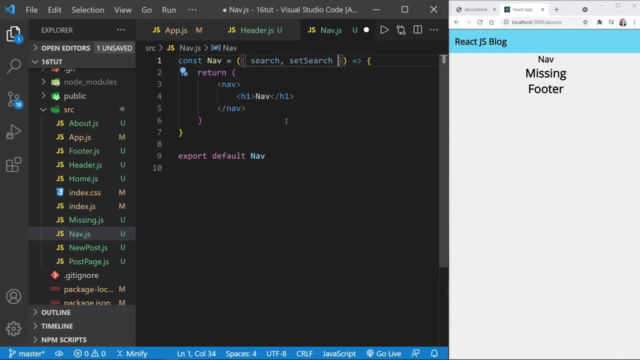 Because we will have a search bar in the nav as well as the links for the menu And instead of an H1. now we do want to have the nav elements, But now, instead of the H1, we're going to have a form here for the search. 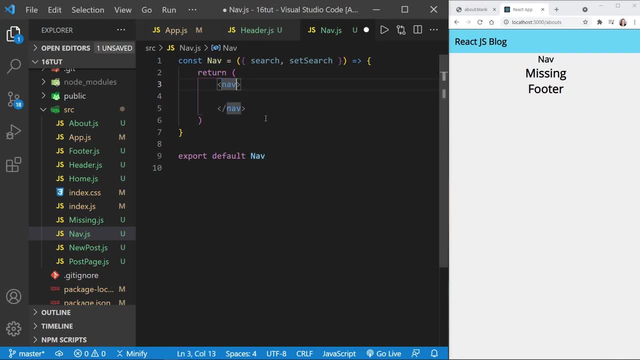 And then we'll also have a menu. Our nav also needs to have a class name attribute And we'll just set that equal to nav. So in the form where we have our search we'll have a class name. We'll set that equal to search form. Going to hide the file tree with control B, as in boy. 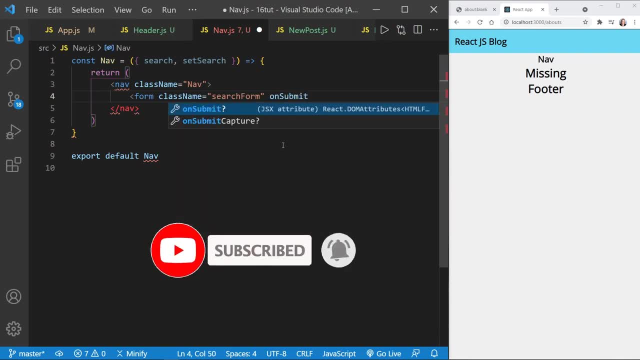 And I can see a little more code now And I'll say, on submit, as we often do with forms, we're going to prevent the default, I believe, And that needs an anonymous function, And then we take the event and have prevent default. 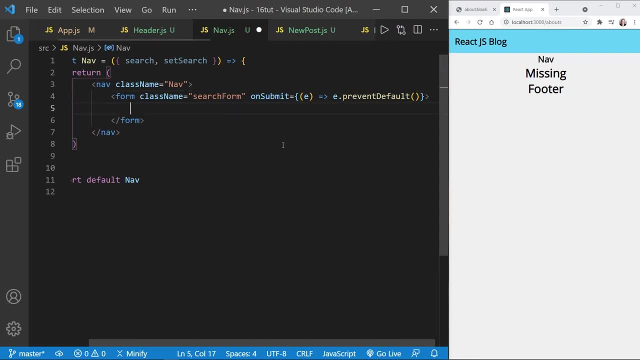 And now we need to close out the form tag. Now we have the closing form tag. We're going to close that out as well. Now, inside the form, we always want to have a label. Even if we don't show the label, we can use CSS to take it off the screen. 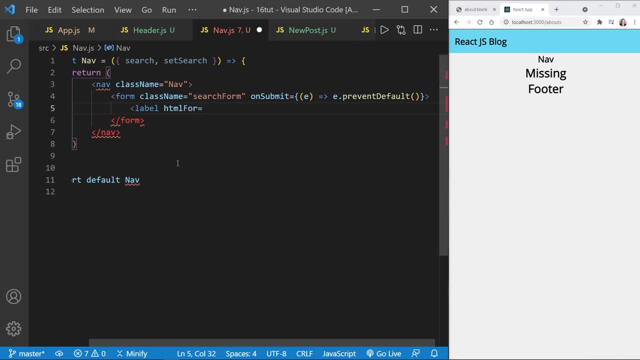 But it will be part of the DOM itself And then screen readers can use it. So we'll just say search here with the HTML4 attribute for the label, And that needs to match the ID of the input And then we can close that. 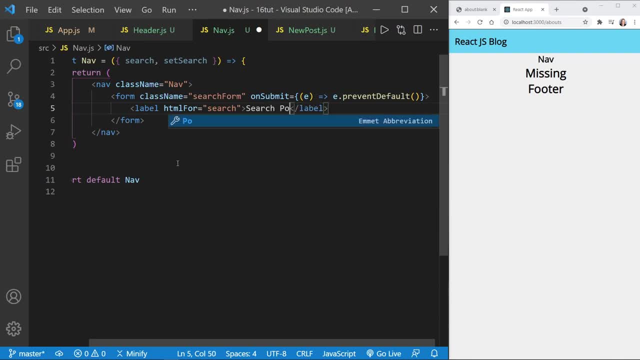 And I'm going to say search posts, because the label just essentially needs to describe what the input does. And then we'll have our input. And now I'm going to put all of the attributes for the input on separate lines. Well, we know we need an ID, that's search. 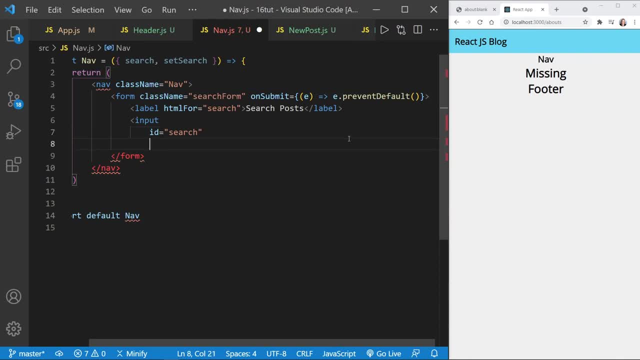 so it matches the HTML4 above. We also want to set the type, And that's going to be a text input, And then we want a placeholder, And this will say the same thing as the label. So we say search posts, And then we'll have a value And we're going to set this equal to. 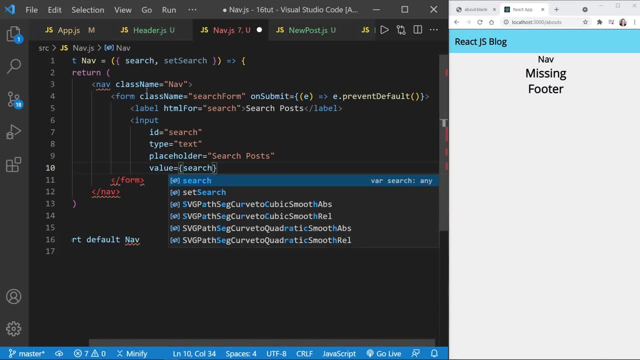 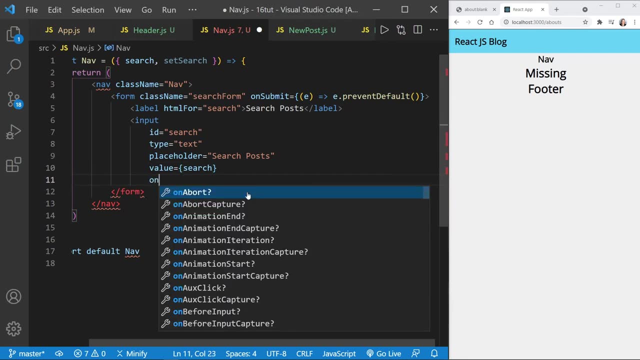 search, And search is what we passed in up here as a prop, So this is going to be a controlled input, And then, just like a controlled input, the onChange also needs to set the search, And we do that with an anonymous function. 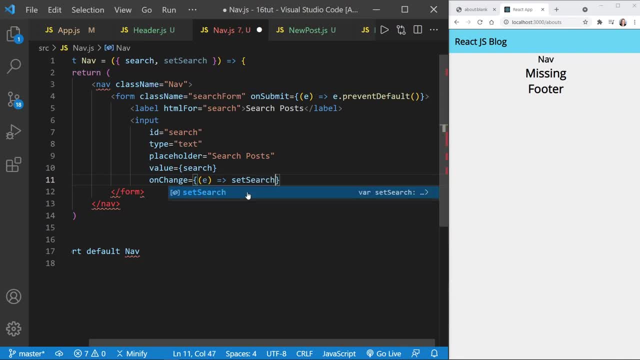 with the event And then we set the search. I have the etargetvalue And that makes this a controlled form input And now we can close that input out And I'll go ahead and bring this back to line it up And we can save that much. Now we're going to have to go ahead. 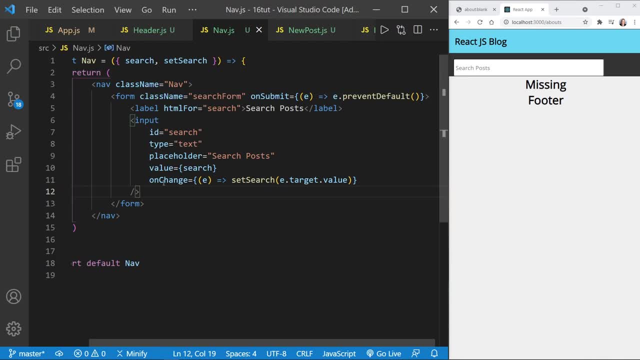 and create the search and set search back in our app to pass those in. But before we do that, we've finished the form. Let's go ahead and create our navigation as well. So an unordered list, And now each list item can be. 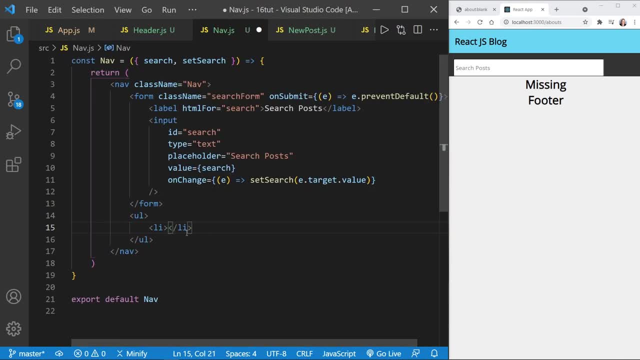 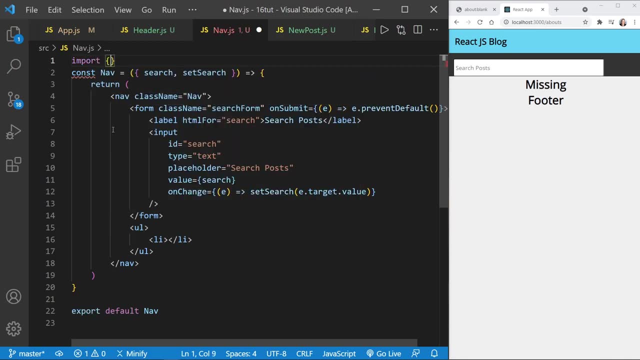 a navigation link, But we haven't imported the link from React Router yet, So let's do that at the top And that's import link from React Router DOM. There we go And we can save that. Now we can use the link as we import it. 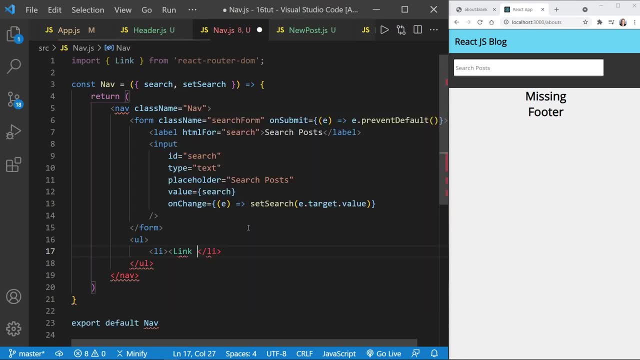 And links render to anchor tags, just like we would see in HTML, like an A with an href. However, this tells React Router: don't request this link from the server, Just route to the proper component. And so now, instead of an href, 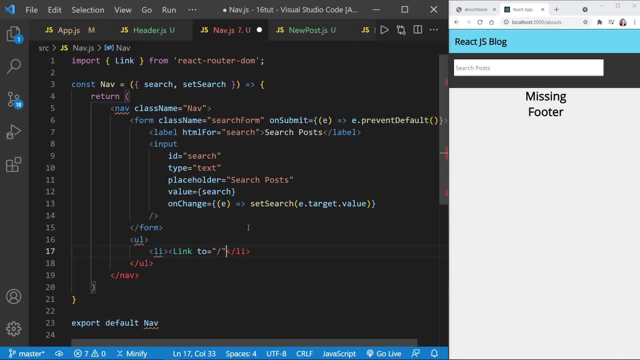 we have a to And we'll set this equal to a slash for our home page. And so there's the link to home, And now I'm going to use shift, alt and the down arrow to make a couple of more links, And now we'll link these. 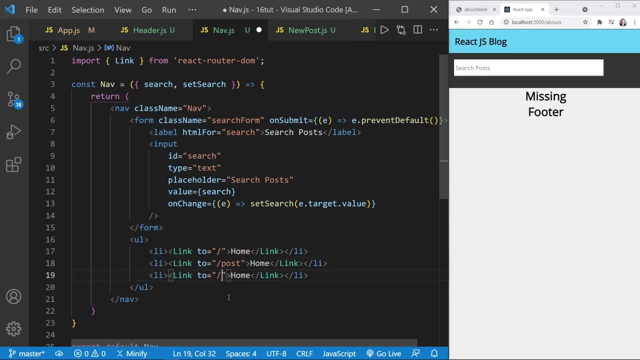 to other pages. So we'll have a link to post and a link to about, And of course we can change the wording here to match post and about, And this will handle the links in our page. So now we save those and we see. 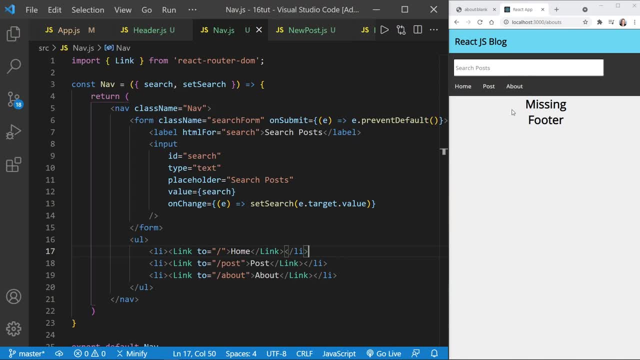 the different links up here. The CSS has already applied itself. So now let me click post- And yes, we went to our new post page. Click home: We're at the home page. Click about: We're at the about page. 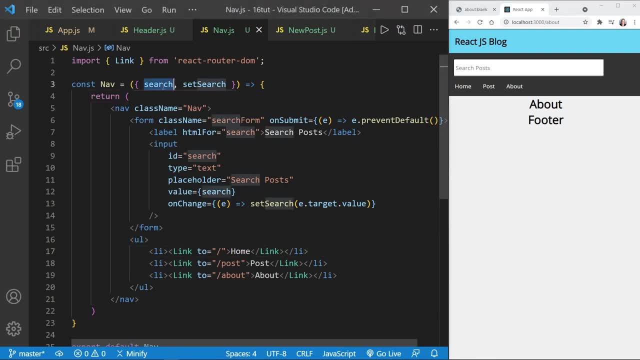 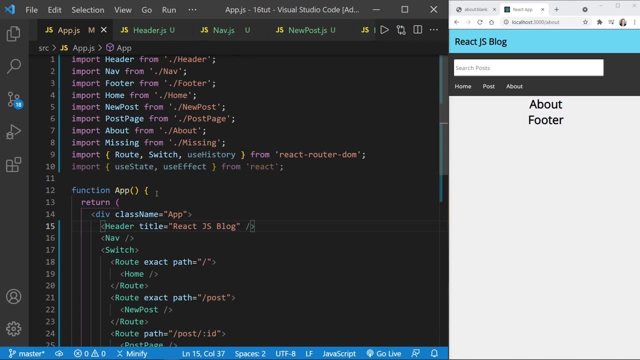 Our links are working. Now we still haven't created our state with search and set search, So let's go back to the appjs and do that very thing. We've got our use state here. So inside the app function we want to define both search and set search. 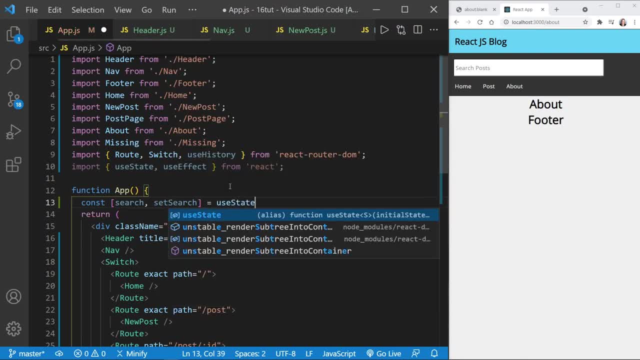 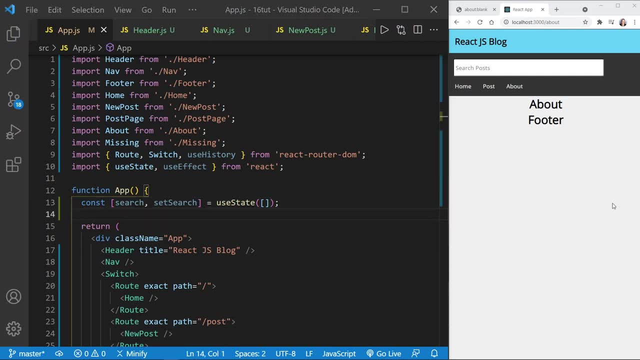 And then we will set that equal to use state And we need an empty array for those as we start out And we'll save that And I'm wrong. I don't want to use an empty array there. I want to do that for the search results. 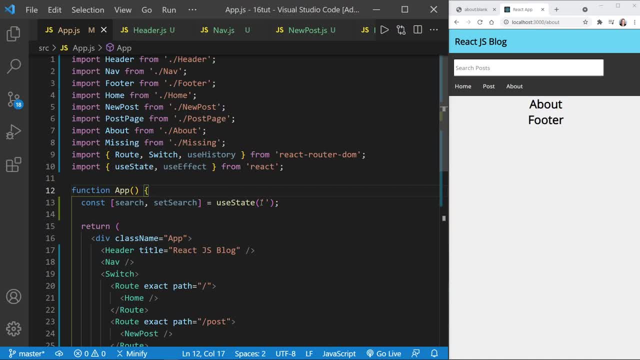 For here I just want to do an empty string. We'll be changing the search string, But then we will have search results that will be stored there And we'll be able to sort it in an array While we're in the appjs and we're creating state, of course. 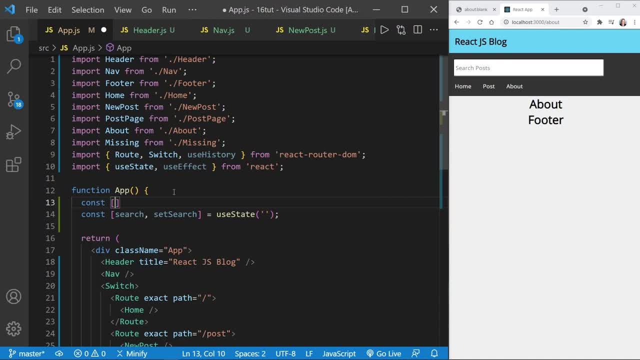 we're going to need some data to search through And for now we will hard code our posts for this dev environment And we can worry about hooking those to an API later. So we'll also have posts and set posts for our blog post. 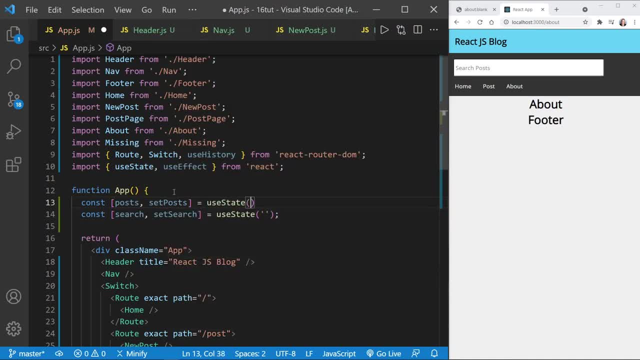 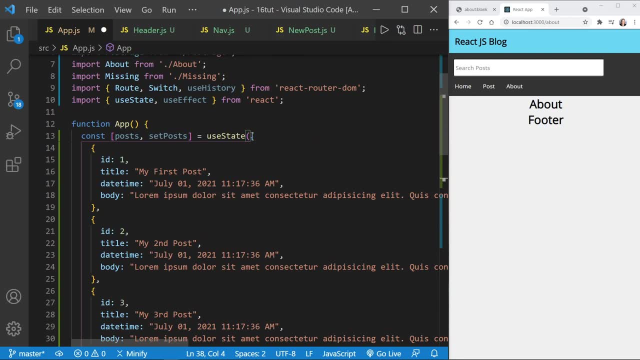 And this will equal use state And this will have an array in it. So I'm going to hard code four posts for now And I'll just paste those in And you can see it's an array. It's an array of objects And each object is a post. 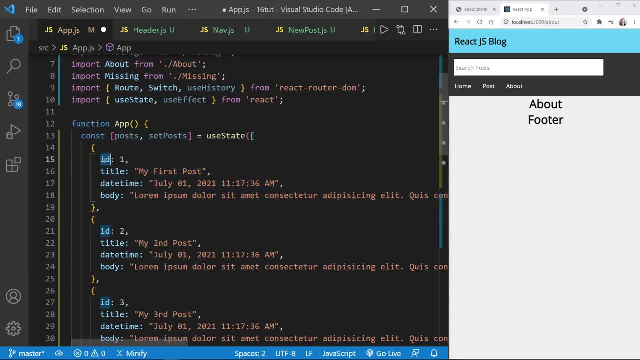 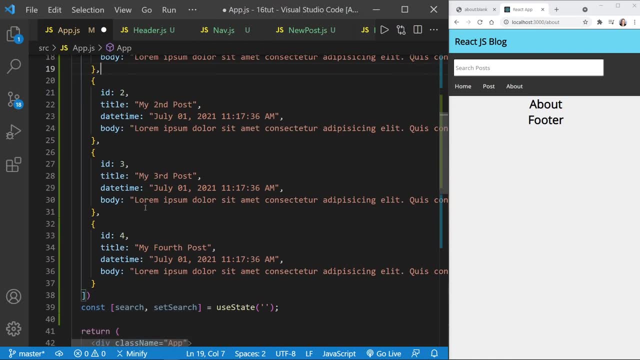 And each post has four different properties. We have an ID, a title, a date, time and a body, And again, this will be linked to in the repository. But you can create your own test post as well, if you just follow this pattern. 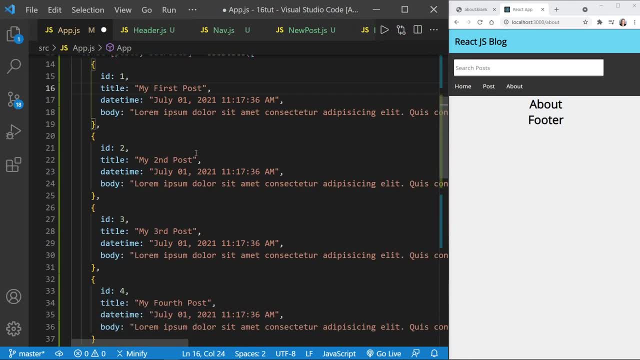 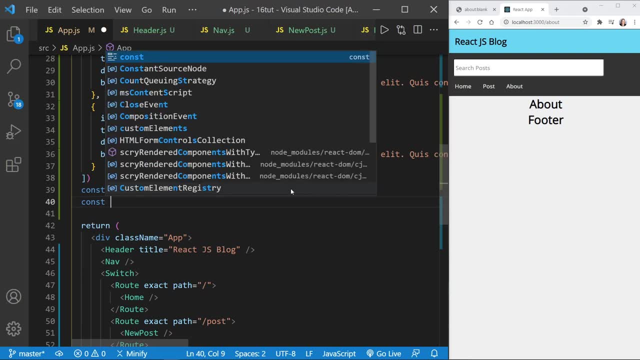 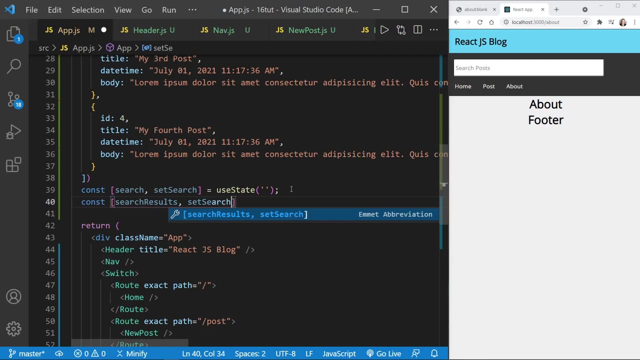 So now we've got posts and set posts using state as well, And we'll save that And let's scroll down And let's go ahead and create the other state I was talking about, Which would be search results, and set search results. 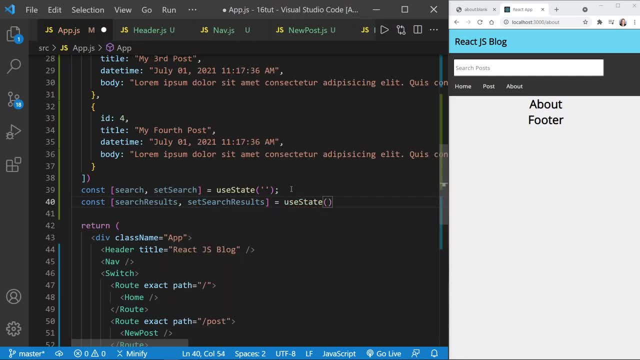 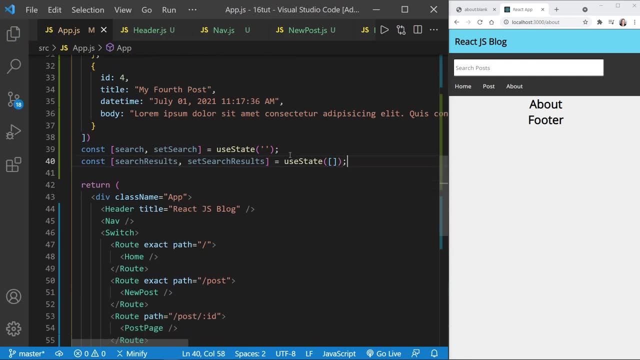 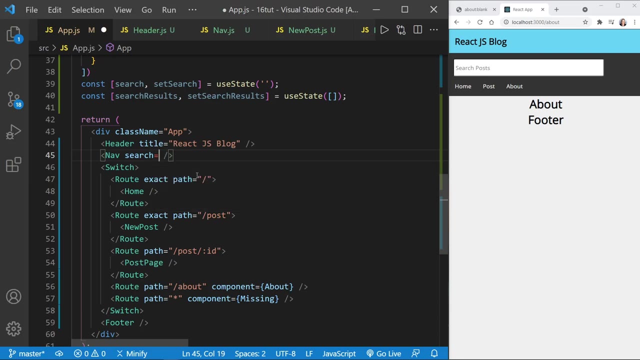 And we'll set that equal to use state And this will also be an array. But we'll just start out with an empty array And we'll save those. Now, if we scroll down just a little bit in our nav component, we need to pass in both: the search equals search. 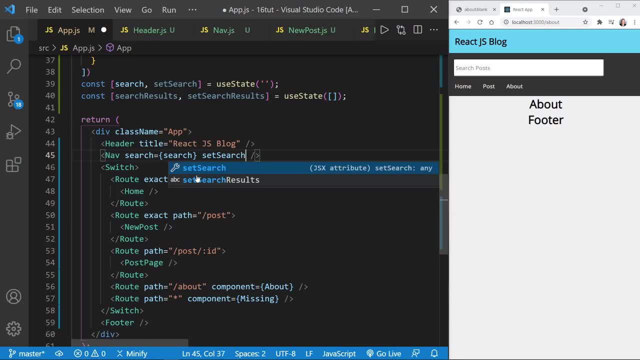 And set search equals set search. And now our nav component is complete And we will be able to search the posts here once we put in just a little more functionality. While we're right here in the JSX, I'm going to go ahead and set posts equal to posts for the home component. 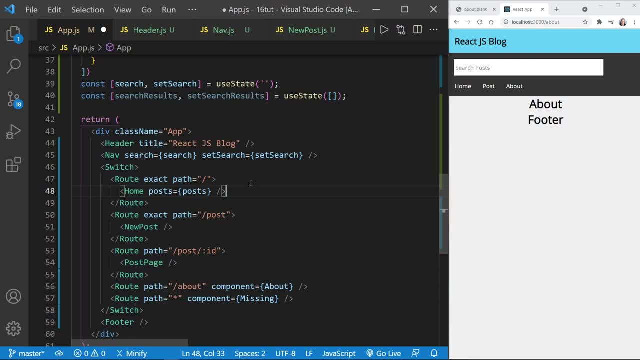 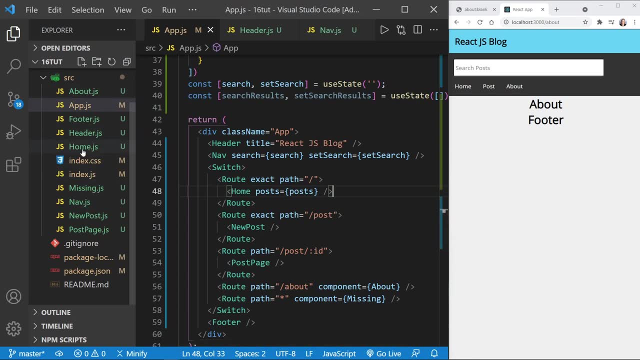 So we'll be passing those posts in because they will display in a feed there. I'll save this and then press control B So I can see the other files over here, And I want to work on the home component. Let's click on home over here with the links so we can see the home component. 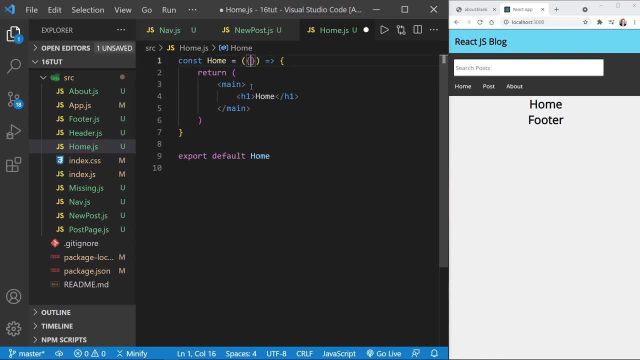 And then it's going to receive the posts And we have the main element here And let's put a class name on the main element. This class name is going to equal home. Let's save that and see if we see a change. 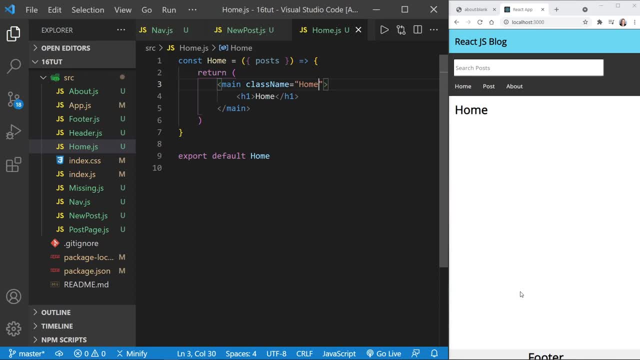 Yes, we do. It now pushes everything down And we see the footer down here at the bottom. So the style for this is set to a flex box And everything in this column should be equal, except the main element has a flex grow value of 1.. 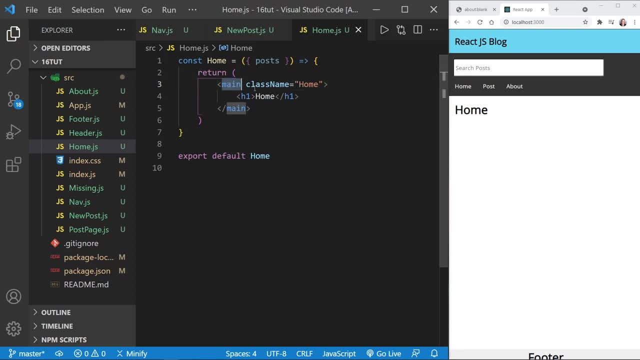 So it grows and fills this out. So when we provide the main element with the proper class, it now fills out our entire page. Okay, inside the H1. now we don't want this home at this point. Or I said H1 inside the home element or the main element. 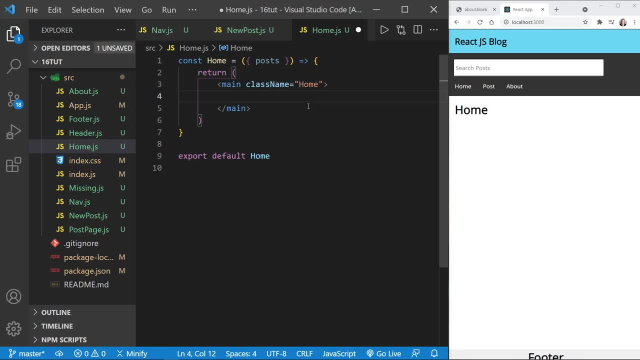 Or the main element of home. We don't want the H1.. We want to actually work with the post to display them, And what we'll do here is check the post's length with a ternary And we'll say, okay, if they have length, now we need a parentheses. 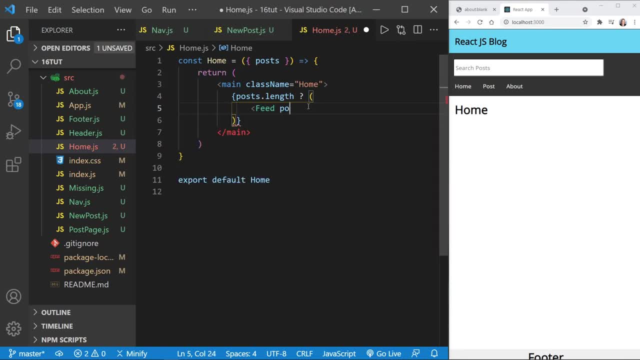 What we're going to do is display a feed component, And this feed component will receive the post as well. So we're drilling those down with prop drilling. If they have length, then we need to do something else here. So another parentheses. 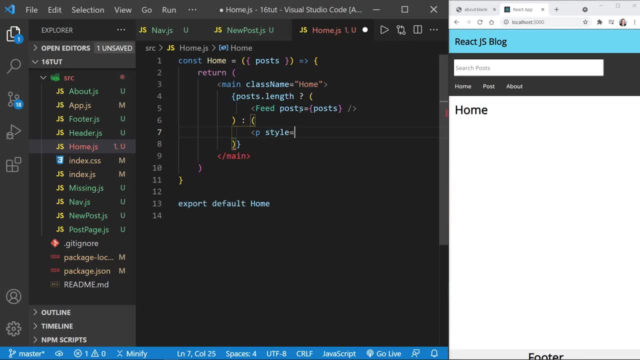 And let's go ahead and put a paragraph here, Set the style, And we'll need two curly braces And we'll give a margin top of 2 rem And then we'll have the closing of the paragraph And on this extra line here we'll just say no posts to display. 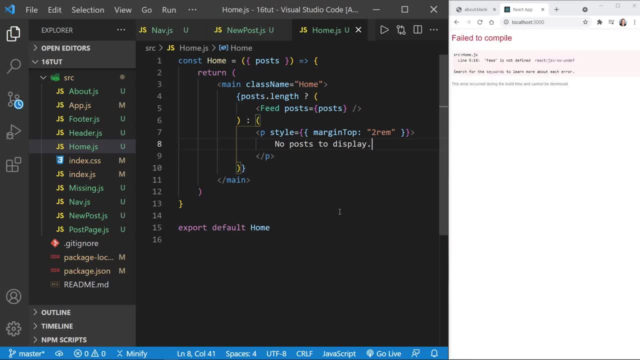 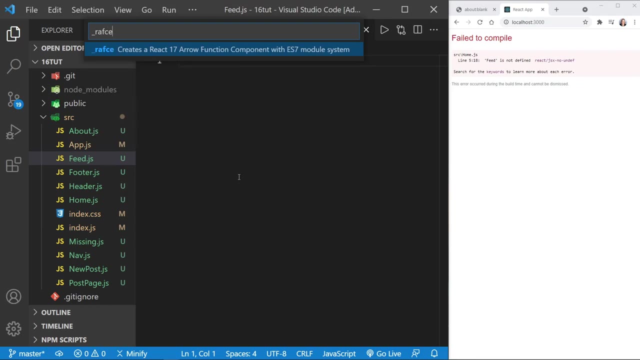 And we can save that, And we might have an error because we haven't created the feed to import yet. So let's go ahead and create a quick feed, component feedjs Inside this. I'll just do Control-Alt-R and then underscore R-A-F-C-E. 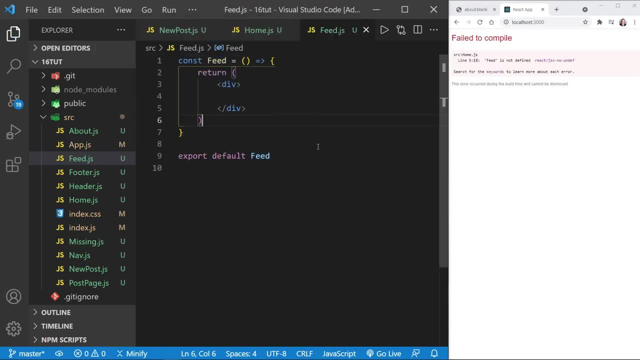 We've created the feed component. It's blank, but that's fine. It will at least eliminate the error. And now we'll go back to home And we need to import before we can eliminate that error. So import feed from slash feed. 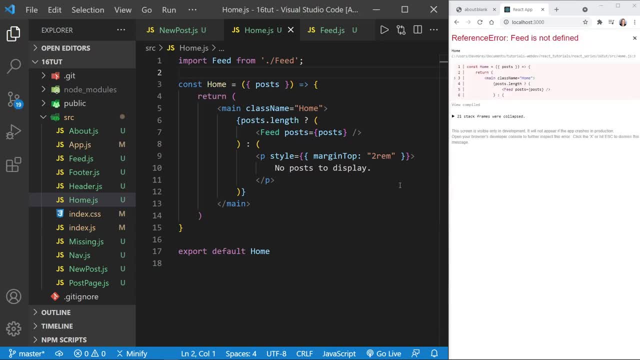 And now the error should go away. Yes, and we just have a blank page because feed is empty. It looks like we have something else. Oh, it says feed is not defined. Let's go ahead and reload and I think it will be all right. 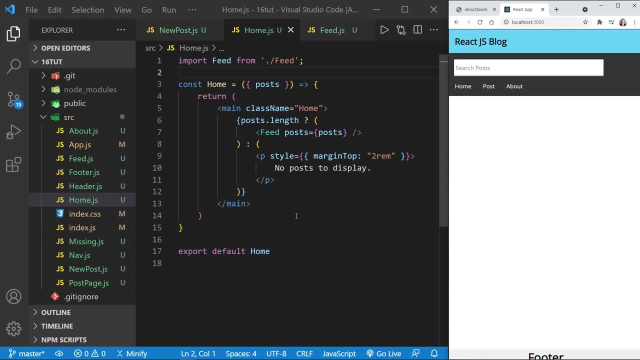 Yes, now we're good, So now we can work on the feed component. Let's click on feed in the file tree And feed is also receiving the posts And, as you might guess, inside of the JSX we need to map through those posts. 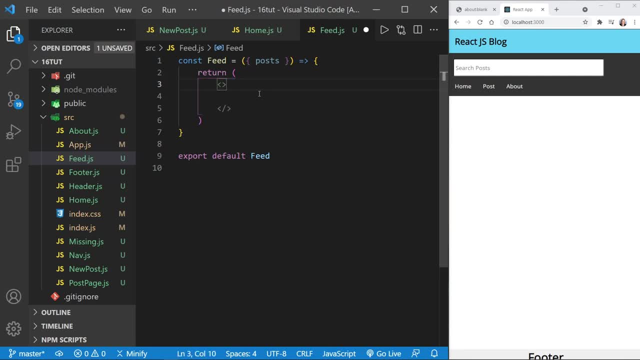 But first let's remove this div and let's just make it an HTML fragment here. So we can do that by just eliminating the words. So we've got the less than, greater than and a slash. So this is just called a fragment in React. 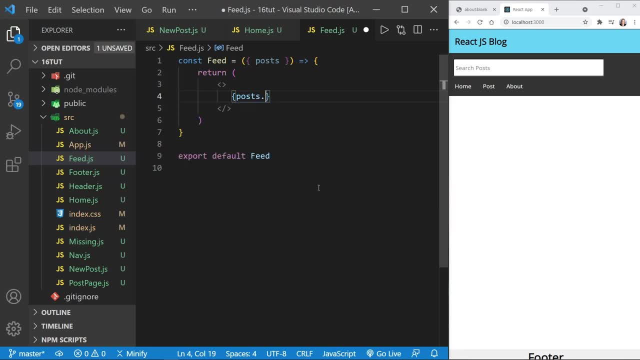 and that works as well. And now we'll have postsmap, and then we map through each post with the arrow, And now we need a parentheses, not a parentheses, not an early brace, And now we're going to use a post component. 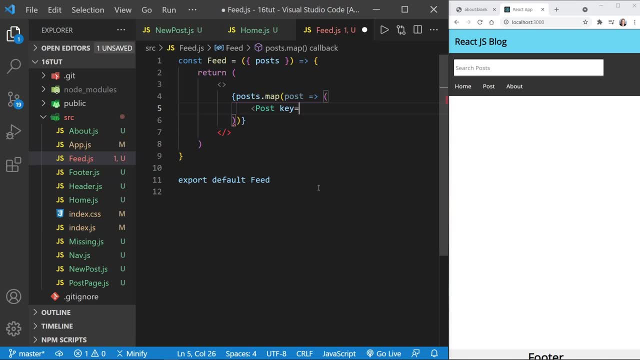 so a reusable component for each post, And it will need a key as you map through, And so that will be the post ID, But then we'll also pass the full post to the component. Oops, not posts, just post. And then we can close out this component. 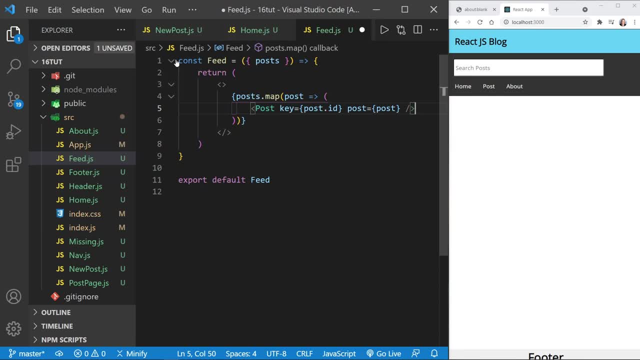 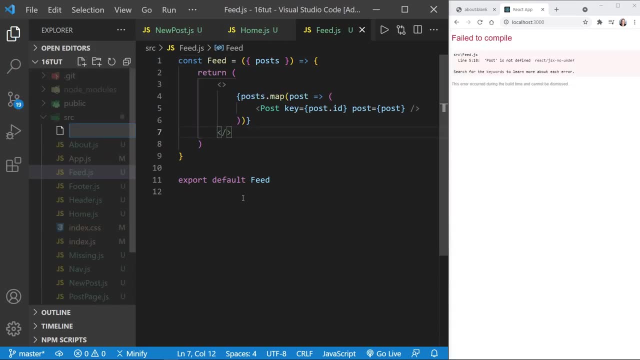 And that's essentially what we need for the feed component here. But of course we're going to need to import post once we create it, So I'll save this and it should create an error again, And then we need to go ahead and create the post component. 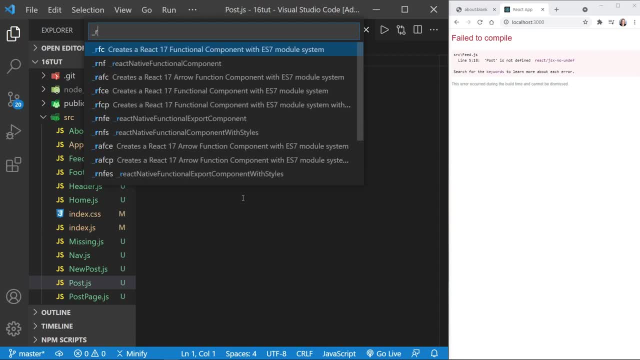 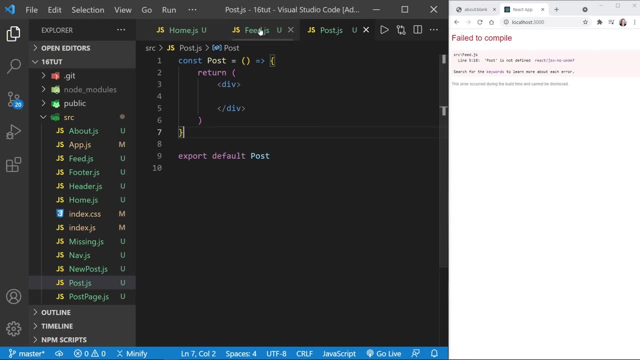 Inside this component, Ctrl-Alt-R, then underscore R-A-F-C-E And we have the post component. Although it's empty, I'll just save it. And now back in feed, we need to import the post. Save that. 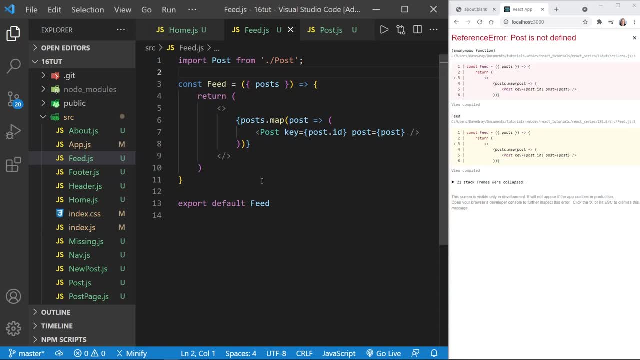 The error should go away, But now it'll still be empty because we haven't done anything inside the post. So now let's work on the post component. In the post component, starting at the top, we're going to need to import link from react-router once again. 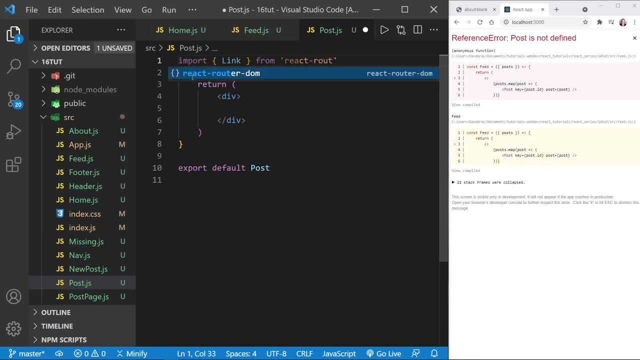 That's react-router-dom. Whoa, it didn't do it. There we go react-router-dom, And now that we have that, we know we're receiving a post. So we need to destructure that at the top. And now we'll make this div an article. 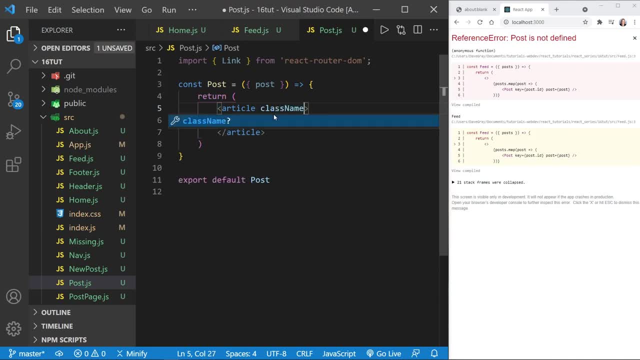 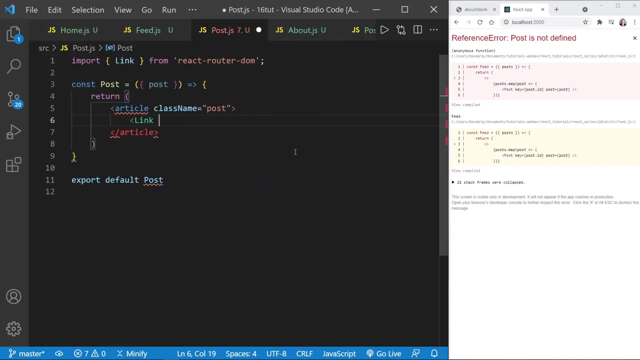 And then we'll give the class name here as well. Class name equals post. And now let's make a link. We want this with a capital L, so it's a react-router-link. I'm going to press Ctrl-D again to hide the file tree. 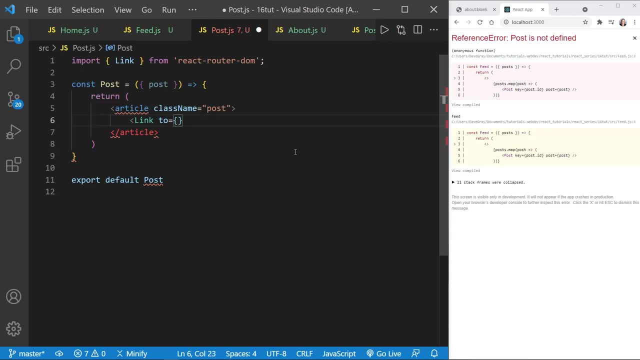 And with this link we'll have a 2.. And now let's make this an expression And we'll use a template link And we'll use a template literal inside, So it will be to the post And then we'll give the postid. 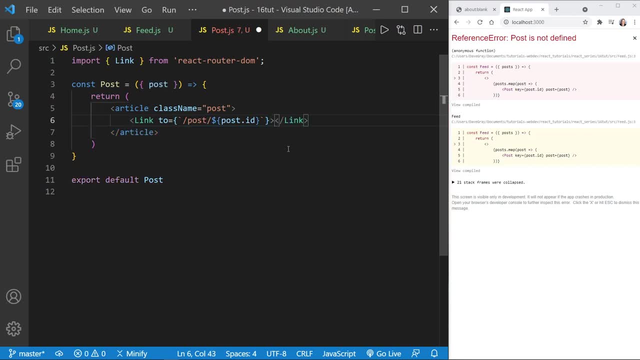 So this will take us to the individual post, And now inside the link we're going to have an H2.. And inside the H2, we'll say posttitle, And then we'll also have a paragraph. We'll give this a class name. 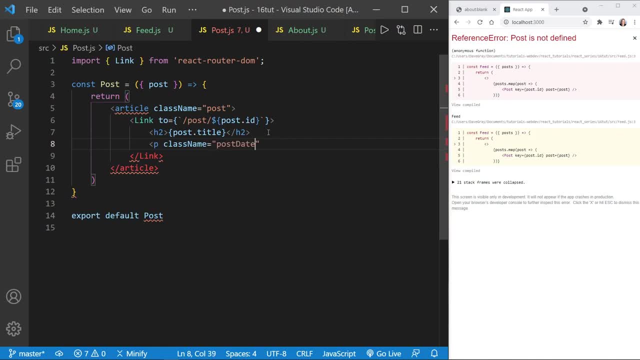 Equal to Post date And this is going to have the postdatetime value that is within each post. And now both of these will be linked to the specific post address with the URL that passes in this parameter of post ID. Now, underneath this link, let's go ahead and give a class name equal to post body. 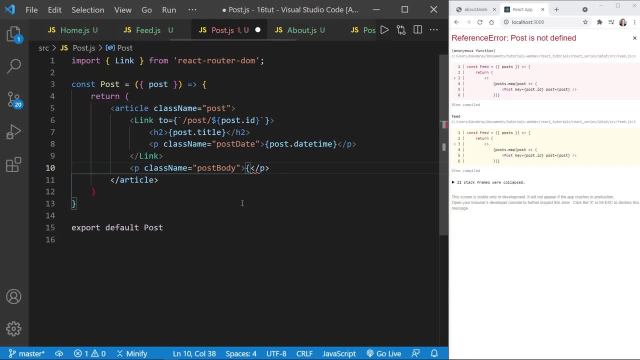 And we'll close that. And now we can give an expression here, And inside the expression we're going to put a ternary statement here. So we'll take the postbody And then we'll get the length of that And then we'll say if it is less than or equal to 25, if that is true, we want to just display the full post body. 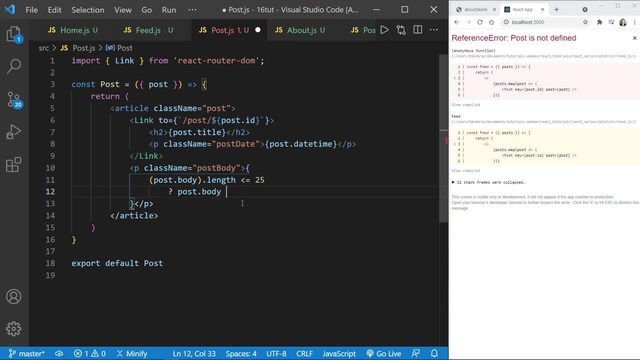 That means the entire post has 25 characters or less. But if it is fullbody, But if it is false, then we'll go ahead and start with a template literal, And then we can have the postbody again And then we'll slice from the postbody. 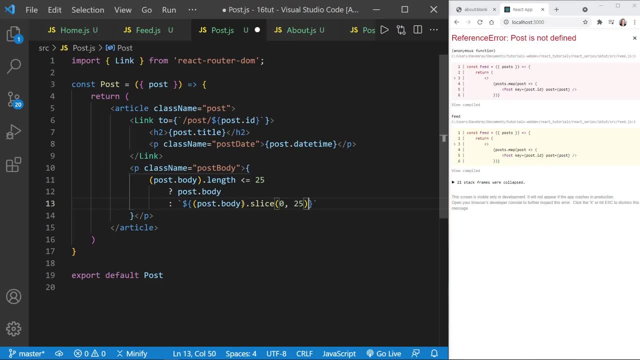 We'll slice the first 25 characters And after that we'll put an ellipsis like three dots at the end, And that way we're only showing a snippet of the full body, Because we don't want any more than 25 characters in the initial feed. 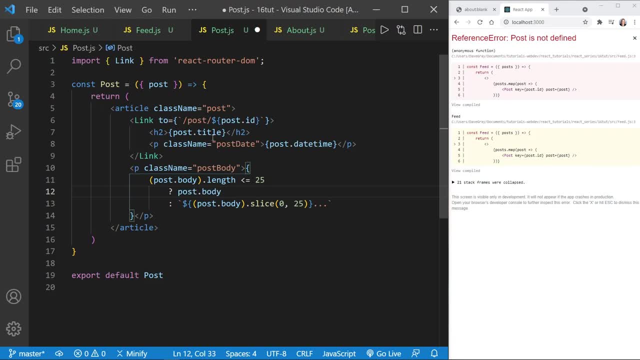 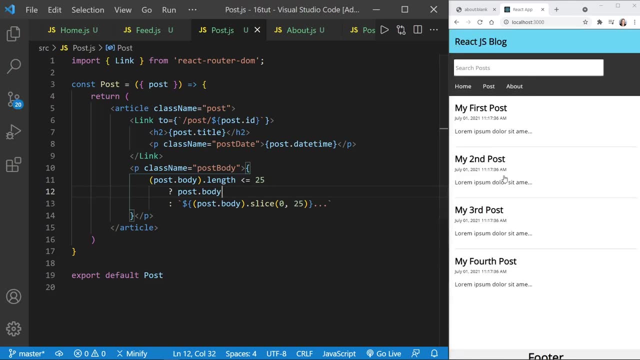 And then you can click on the full link above here and see the full post. So let's save that. And now we can see our feed with each post, And of course, I've used Lorem Ipsum in each one of them, And so they're all the same right now. 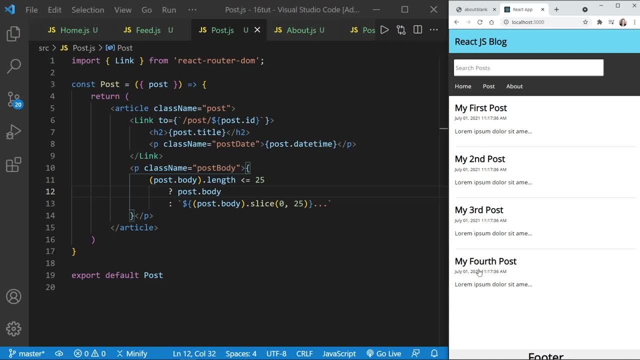 But we see they go the first 25 characters And then we get that ellipsis And this should be linking to each individual post. So if I click my first post, Yes, it takes us to the post page That we haven't designed this component yet. 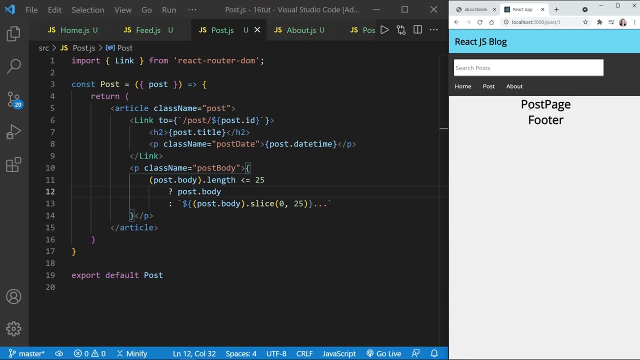 But that should show the details and the full postbody for the individual post that we're supposed to see, as it grabs the parameter out of the URL. So let's work on this post page now. I'm going to press Ctrl B to show the file tree. 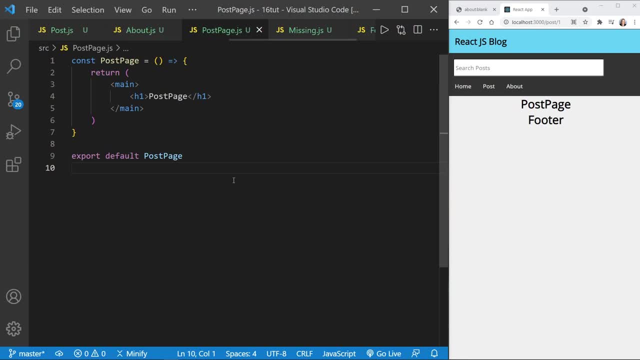 Select post page And I'll press Ctrl B once again to hide the file tree. Now inside the post page, we're going to import a couple of things at the top, So let's just do that right away: Import destructure here. 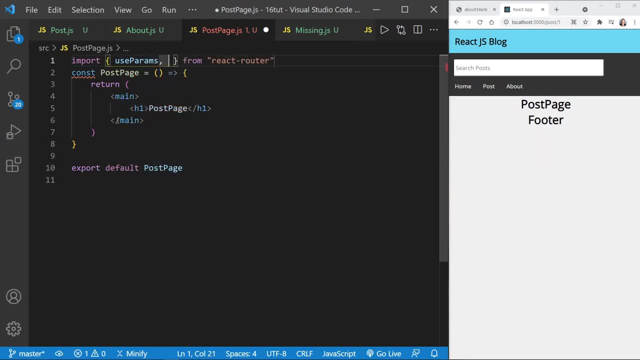 And we're going to import use params, Which is a custom hook that comes with React Router DOM, And we're also going to import link, But it just says from React Router. I don't know why it's saying that. So we also want it to be from React Router DOM, here at the top. 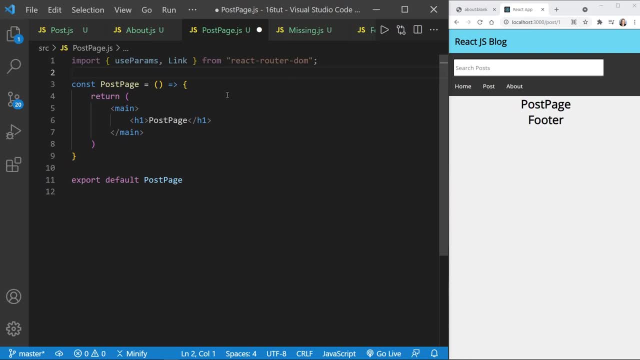 Okay, once we've got those imports ready to go, We're going to receive a couple of things as props. One, of course, is the posts. The other is going to be a handle delete function, Because we're going to offer a delete button on this page as well. 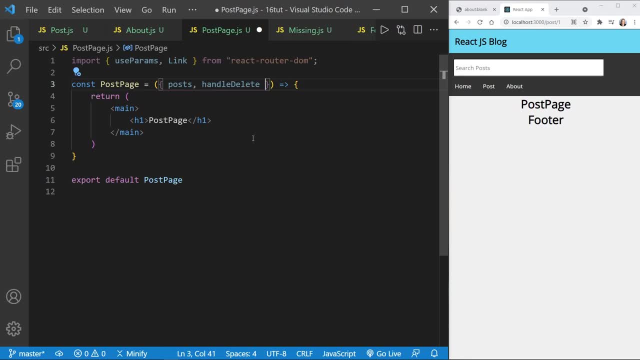 So those are the props coming into the page, And now let's go ahead and define the ID inside the function, And this is going to be equal to use params. And we said ID here because that's what we called it in our route back in AppJS. 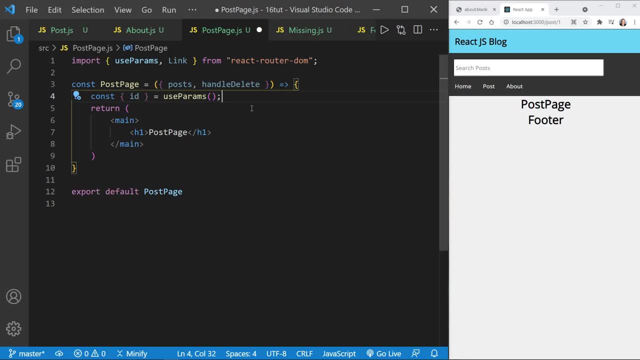 When we defined the parameter for post page. So that's what you need to do. If you named it something different, You need to also have this named differently. So that's what's defined in the route. And then, once we have the posts here, 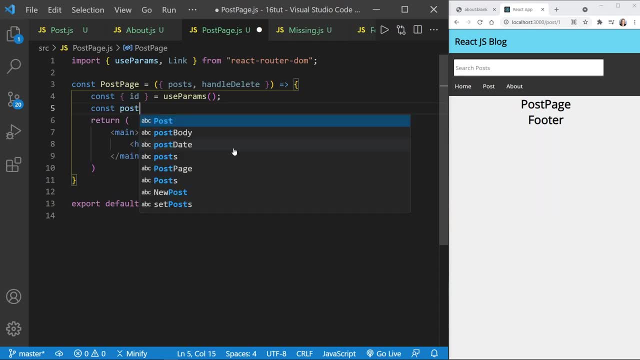 We need to get the individual post we want to display. So let's say post equals postfind. And now we get the post And here we'll take the postid And then we'll set it to a string, Because it is really numeric. 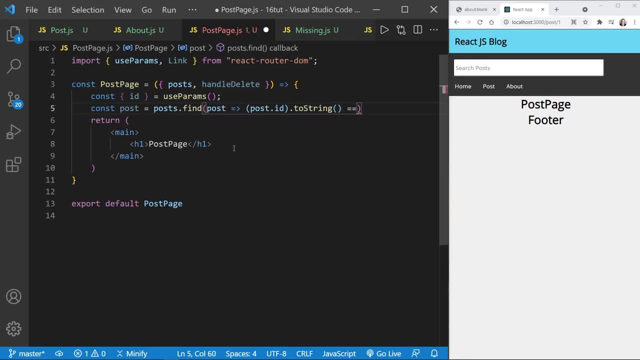 So if we didn't set it to a string, We would only be able to use two equals, Which you could also do if that's your preference. I prefer to use strict equals when I can, But in order for me to do that here, 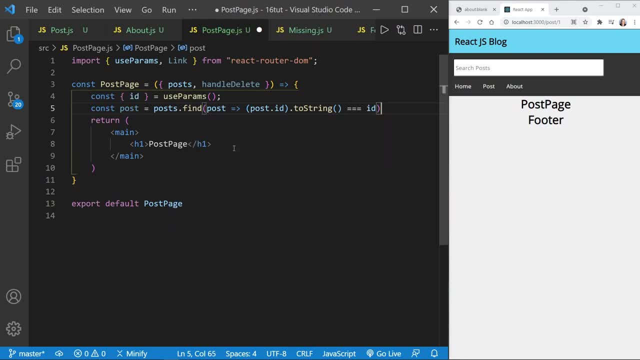 I need to set that to a string to match the ID. That is also going to be a string coming from the parameter. So, once again, if you don't set this to a string, You'll need to go to non-strict equals, Just the two equal signs. 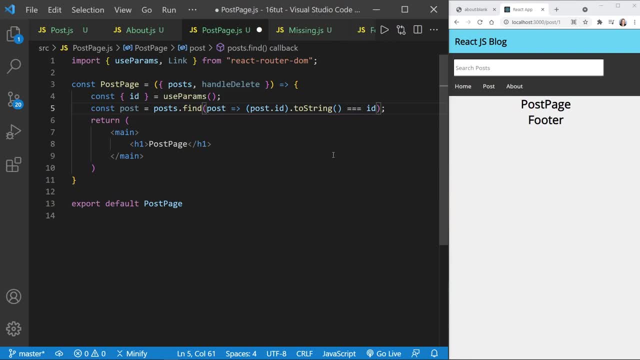 So it's up to you. Whichever you do, This is the way I'm doing it, And we've defined the specific post that we want to see now. Now, with the main element here inside the JSX, Let's set the class name equal to post page. 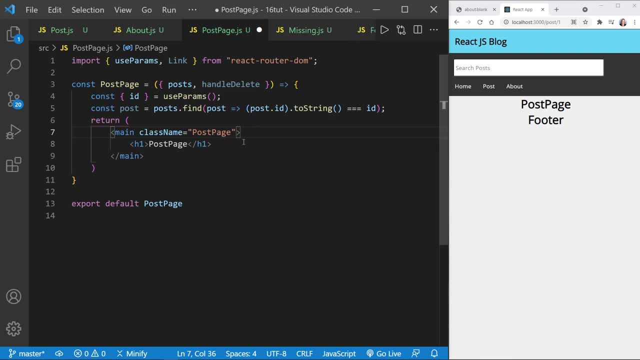 And then after that, we're going to have an article And let's give the article a class name equal to post. Let's go ahead and get rid of this h1 element. And now, inside the article, It depends if we have a post display or not. 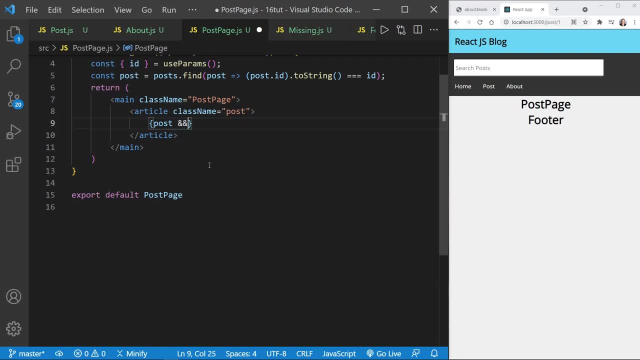 So let's say, if we have a post And then use the two ampersands, Which is a way of saying okay, If the post is true, Essentially if it exists, Then we're going to display this And inside of our curly braces. 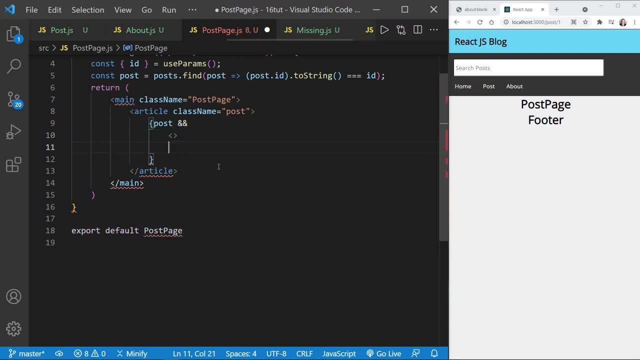 After the ampersand Let's put a fragment once again, And so now that we have a fragment for the parent, We can put our other elements. So we'll have an h2.. And inside the h2. I'm going to say post dot title. 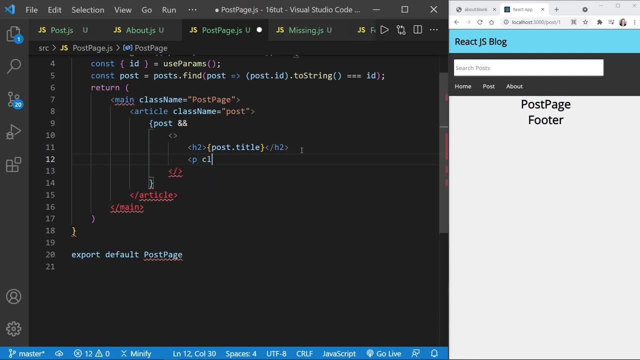 And then the next one will be a paragraph with a class name, And here it's going to be the post date, And inside this, of course, we'll put post dot date time. And now I'm just going to copy down with shift, alt and the down arrow: 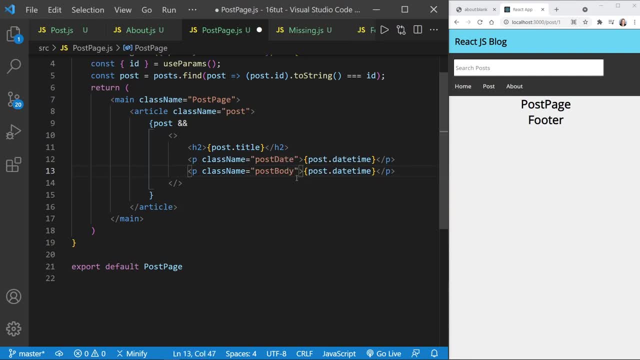 Change this post date To post body, And here, of course, it will be post dot body. And then, finally, we need our delete button. So this will be a button And let's give it an on click. Let's set this equal to with a curly brace. 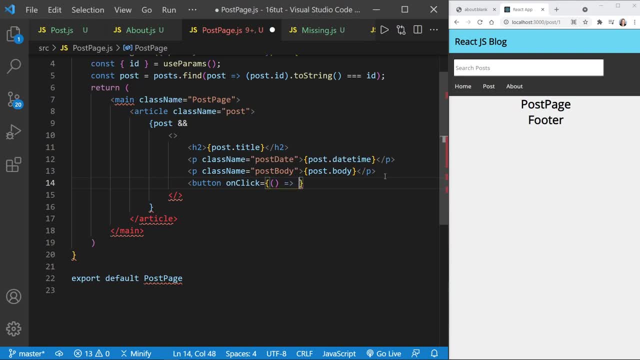 And then we get an anonymous function And inside the anonymous function We're going to call handle, delete, But we need to pass in the post id And then after that we can close out the element And display on the button. We can just say delete post. 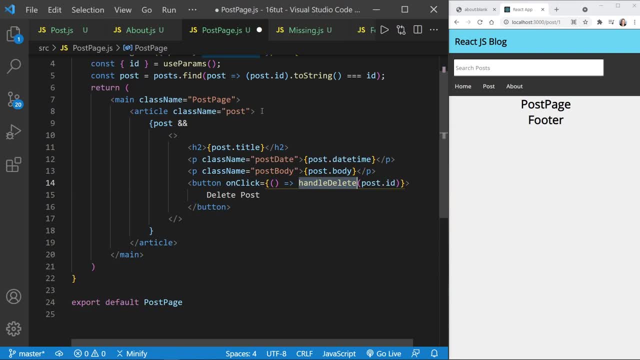 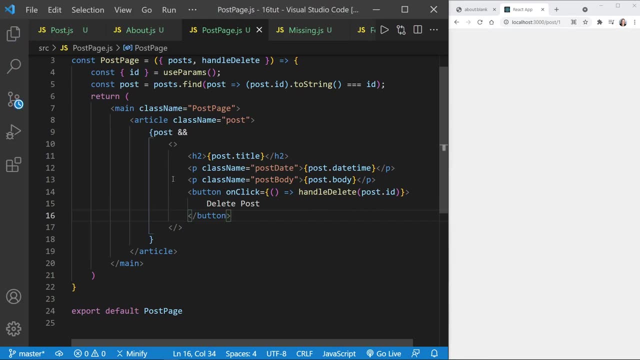 So now we know we need a handle delete function. That is coming in as a prop And it receives an id, So we can save all of this. But we're not quite finished yet. Oh, and something is undefined. Cannot read property find of undefined. 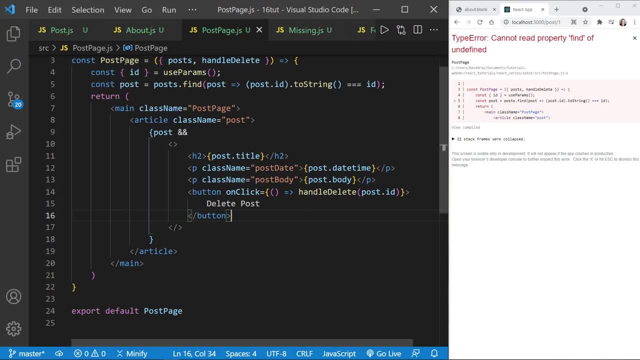 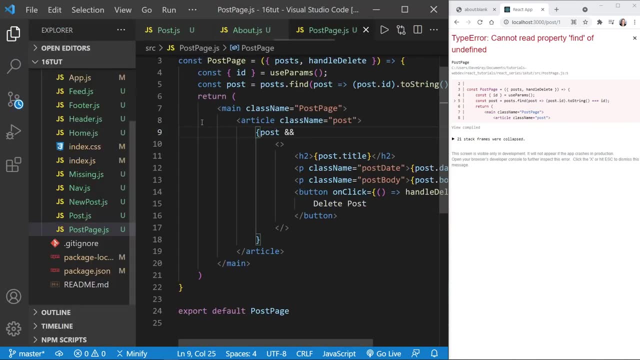 And I believe that is because we're not passing anything Yet to post page from the app js. Well, that's not it. Let me go ahead and show the file tree. Click on app js And if we come down here to post page, 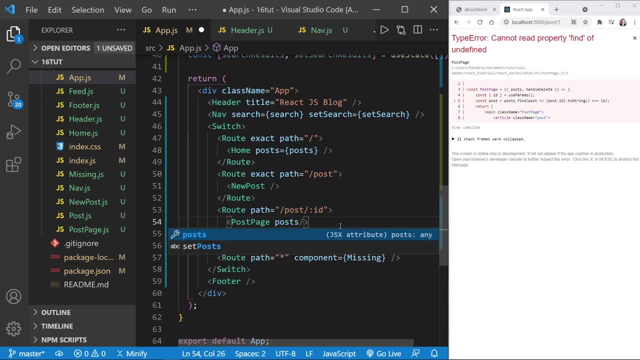 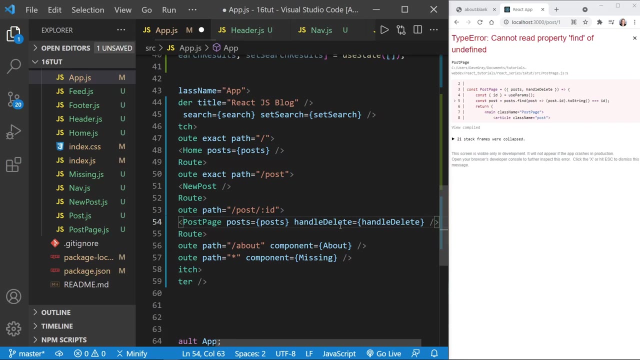 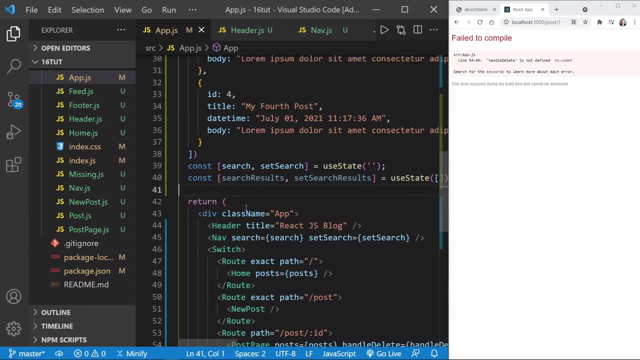 We haven't passed in those props yet. So let's say posts equals posts And we're also going to have handle delete equals handle delete And save. Now we'll probably still have an error Because we haven't defined handle delete. Let's just come up here to the top, above the return. 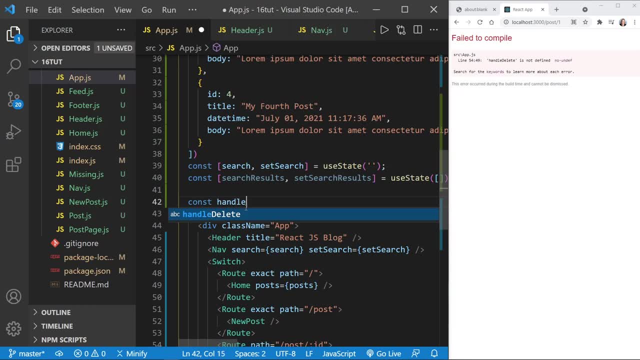 And we're in the app js, We'll quickly define, handle, delete And then we can add more details later And we'll just put details in here a little bit later. I believe empty is okay for now. Let's see if we get past that error. 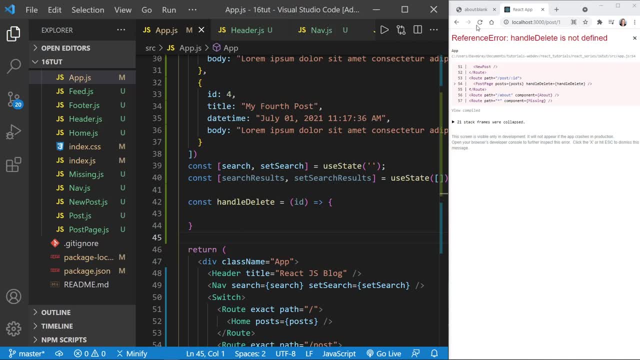 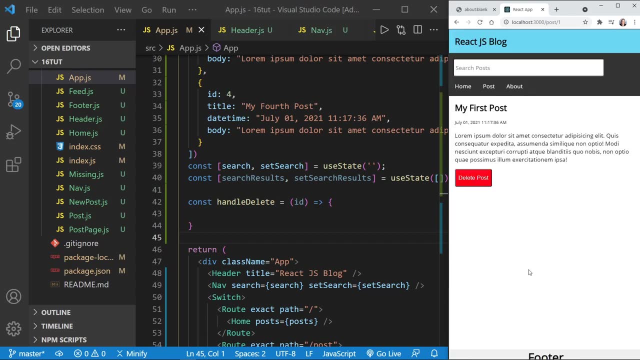 Yes, we're past it And we got a display. Let me go ahead. And it says: handle delete is not defined. I think it just needs reloaded. Yep, And now we're good, Back in the post page, though We haven't quite finished our definition yet. 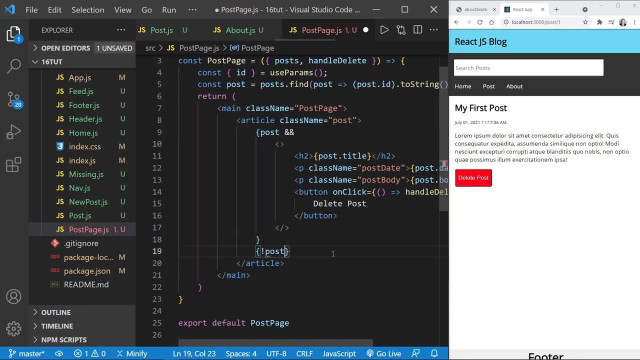 Because what if we don't have a post? So we need an option if post is not true. Essentially, with the exclamation mark here It does not exist, But we've somehow got to this page. I'm just going to quickly paste in what I'll put here. 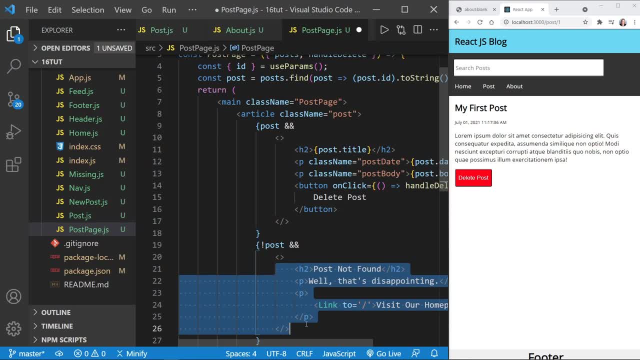 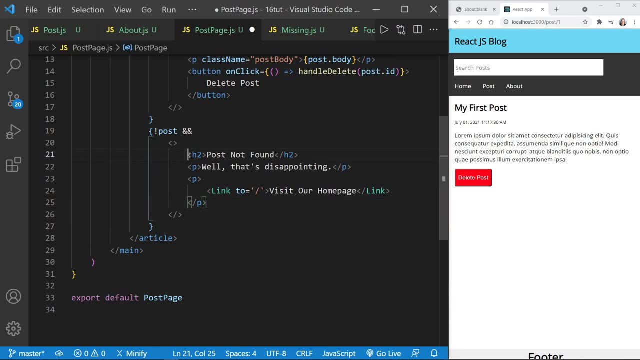 And you can see we have an HTML3. HTML fragment. once again, As we use in React, I'm going to hide the file tree so you can see everything. And inside the fragment we have an H2 with post not found. And then I just say, well, that's disappointing. 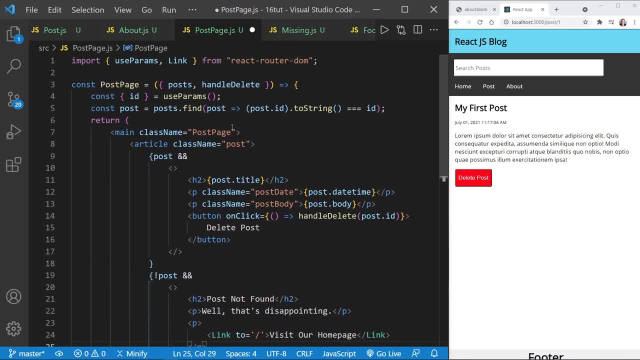 And we put a link that says visit our home page, And so that's why we've imported link above as well. And so now we're using the use params from React router to get the parameter And we're using link to provide a link back to the home page if it doesn't exist. 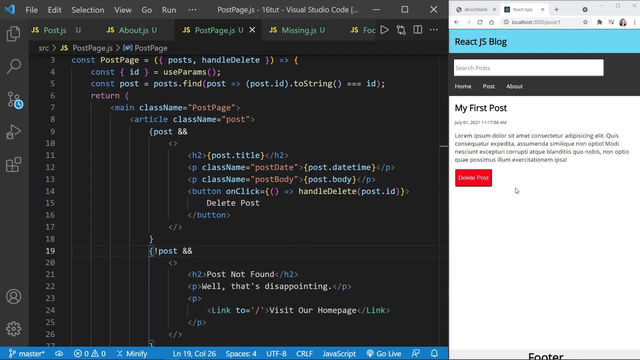 So let's save this And you can see use params is already working. We wanted my first post, and that's what we got. If we switch this to number four, We should get my fourth post, And that's what we got as well. 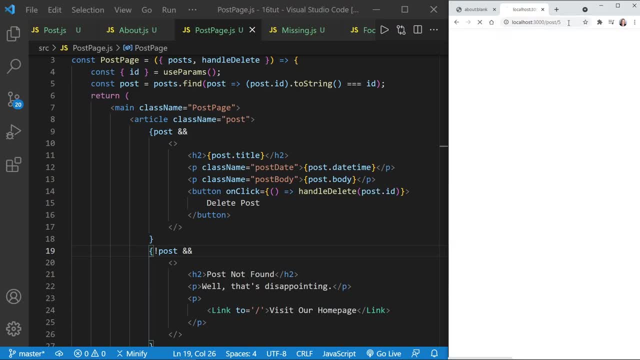 But if we go ahead and request post number five that doesn't exist, We get our portion here where the post doesn't exist And it says post not found. Well, that's disappointing. Visit our home page And the link works. I'm going to press control B to show the file. 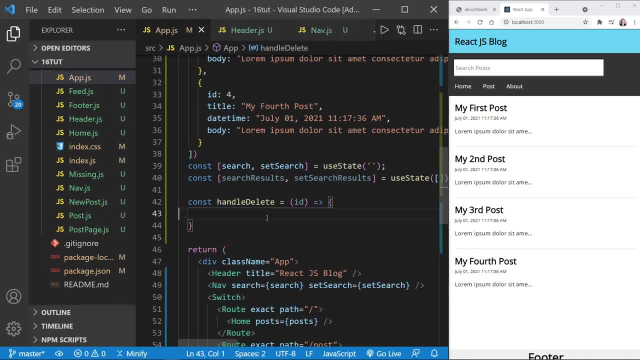 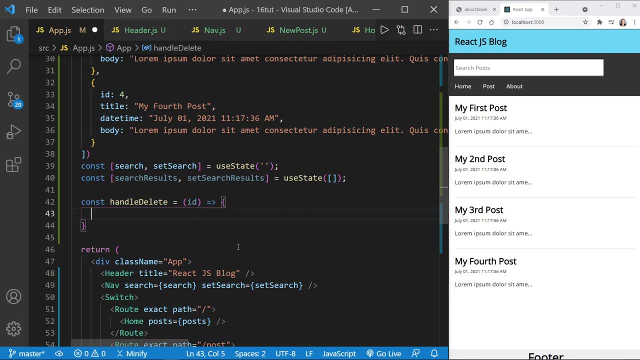 Tree, again Go to appjs, And now we need to go ahead and finish defining our handle delete function. What's going to happen is we receive the post ID here, So then we can just define our posts list, And we'll set this equal to posts dot filter. 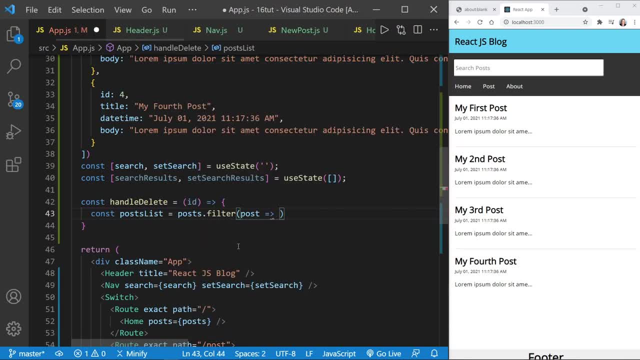 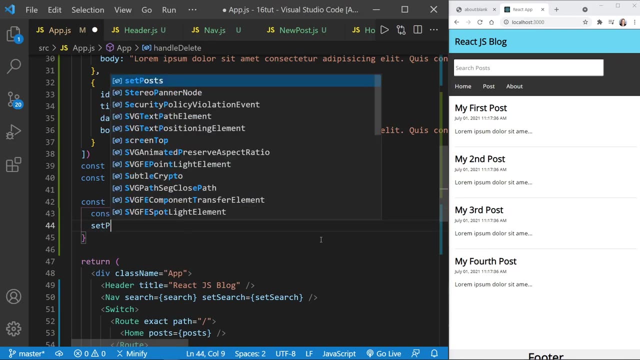 And there we have a post, And if the post dot ID is not equal to the ID, Then we'll include it in the post. So we're filtering out the post that has the ID that we have passed in. From there we can just set posts back to the new posts list. 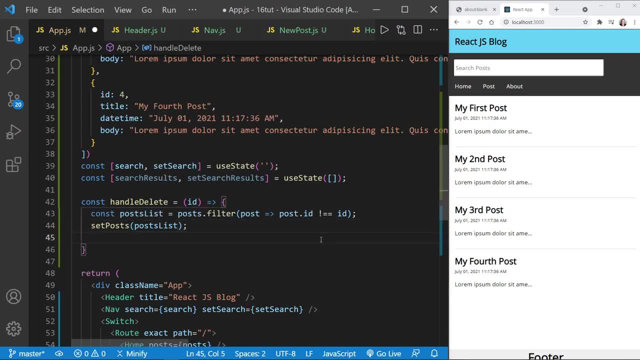 That doesn't have the post with that ID. And now we want to use our browser history. We click the delete button, But we're on the individual post page, So we can do that with the use history hook that we are importing up here. 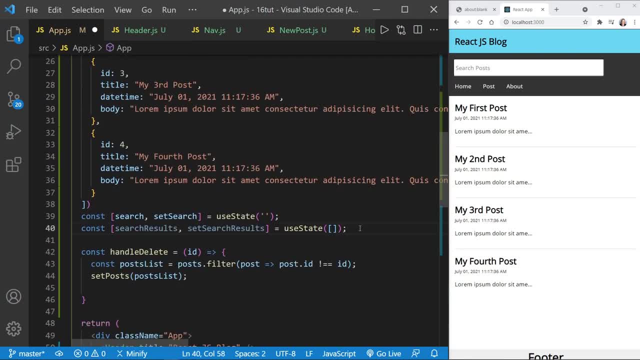 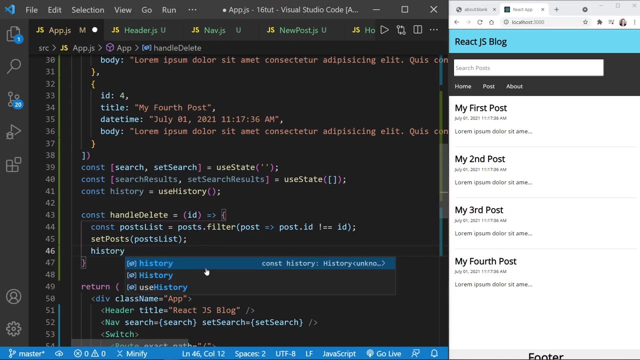 Now, underneath where we set the use state, Let's go ahead and hit return And we'll just say history is equal to use history, And after we've defined that, we can use it inside of our handle delete function. So we'll say history dot push. 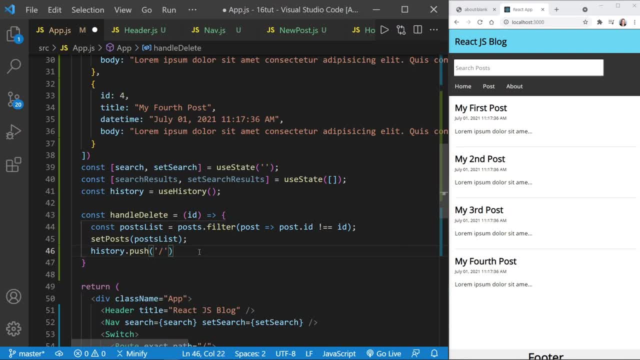 And we'll just push in the route to the home page And this will take us back to the home page once this is completed. So, as part of the function, we're accessing the browser history with react router And then we're serving the component instead of requesting anything from the server. 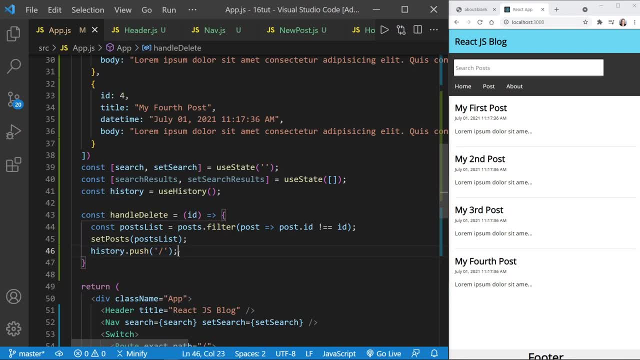 We're serving the component that is routed to that home directory listing. With this saved, let's go ahead. We've got our posts over here on the right in Chrome. I'll click my third post. Here's my third post. I'll click delete post. 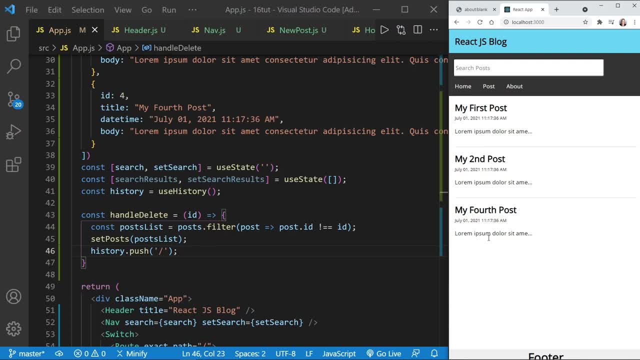 It deletes the post and takes us back to the home page instantly And notice there's no third post Now because we have hard coded our posts in our state. When I reload the application completely, we get my third post back. So you can play around with this and delete them right now and they will come back. 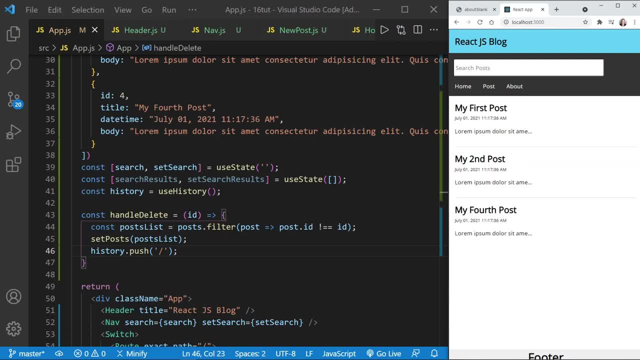 But everything looks and works as it should. We now need to work on the new post component that we will see when we click post. That allows us to create a new post, But before we do that, we need to create some more state inside of our appjs that we will be using inside that new post component. 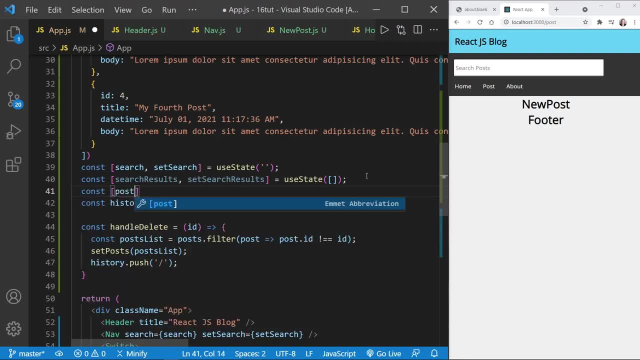 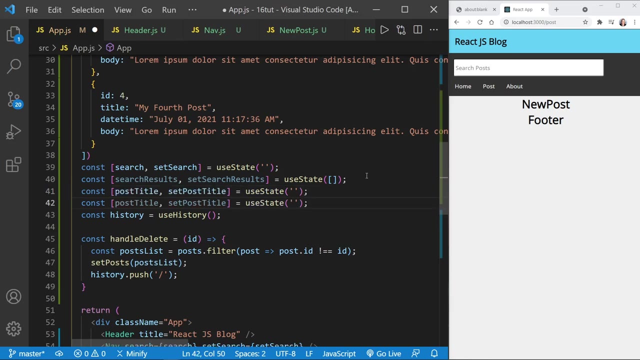 So we'll say const, And here we're going to have post title And set post title And this will be equal to use state And this should be an empty string And then I'm just going to copy that down And we'll also have post body and set post body. 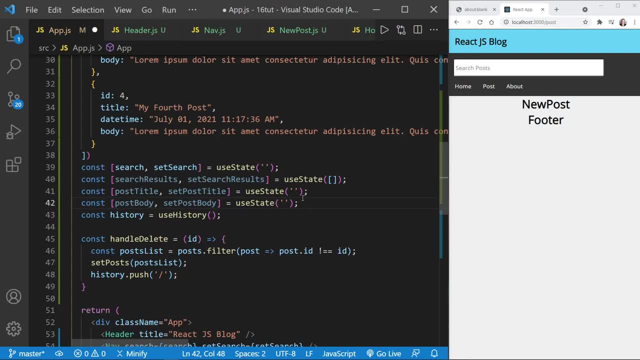 So I'll change those to body And that's also equal to an empty string. And now that we've defined both of those, we're going to pass both the post title, post body and the set post title and set post body All in as props to our new post component. 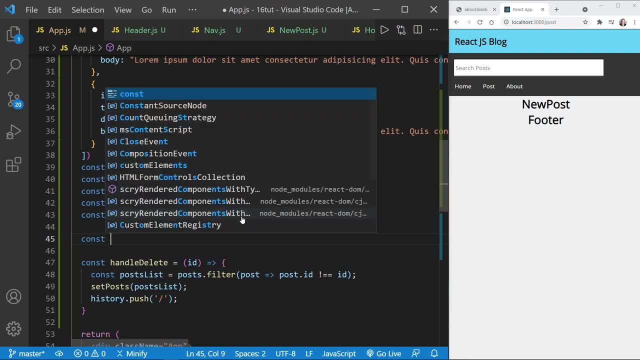 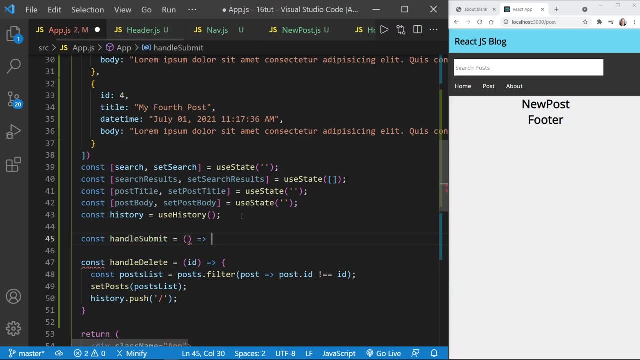 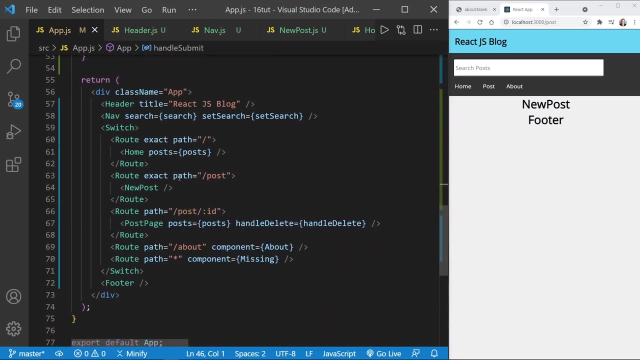 But we also need a handle submit function as we submit a new post. So here is our handle submit And we'll just make an empty function right now, once again, And come back and define it when we're ready. Let's go ahead and scroll down to our JSX, where we can pass all of these props into new post. 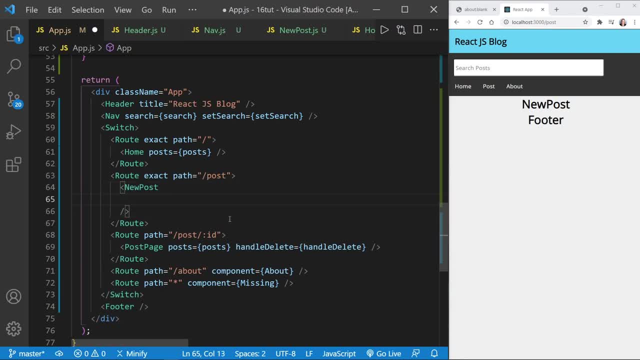 So it's receiving more than most of our other components, Or it is receiving more than all of our other components actually. So we'll have: handle submit is equal to handle submit. And then, on the next line, we're going to go ahead and have post title is equal to post title. 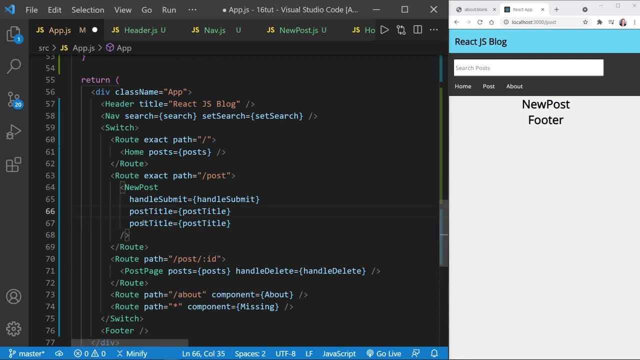 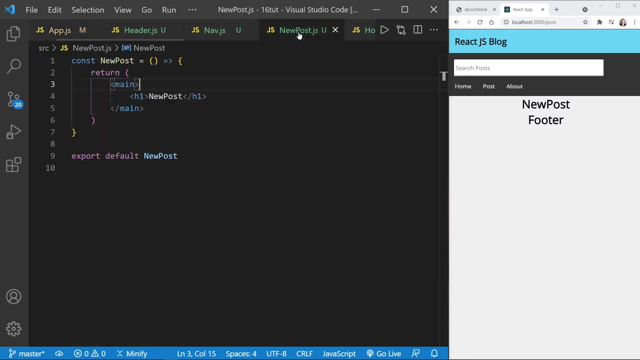 We'll copy that down And then we're going to have set post title is equal to set post title. We'll have post body equal to post body And finally we're going to have set post body equal to set post body. We'll save those and we'll go straight to the new post component to begin adding everything we need to it. 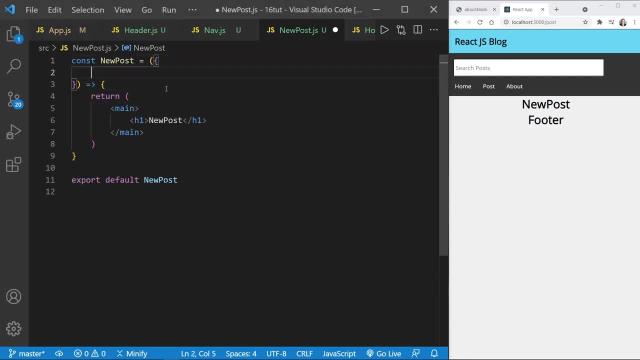 Inside new post. we've got a lot to destructure as we pass in all of those props, So I'm going to add it on an extra line here. Say handle, submit, And then we've got post title, set post title, post body and set post body. 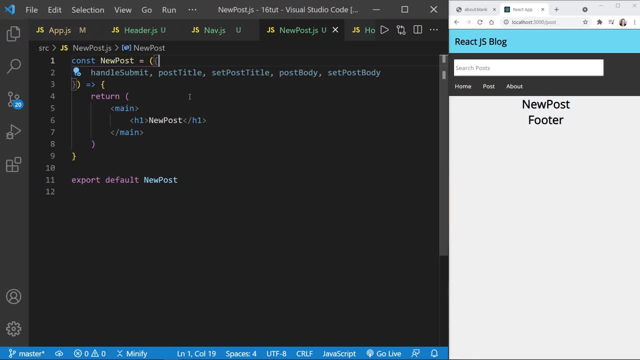 All coming in as destructured props. I'll save that And now we're ready to go ahead and add a class name to the main element. I'm going to set this equal to new post And if we save, we should see a change. 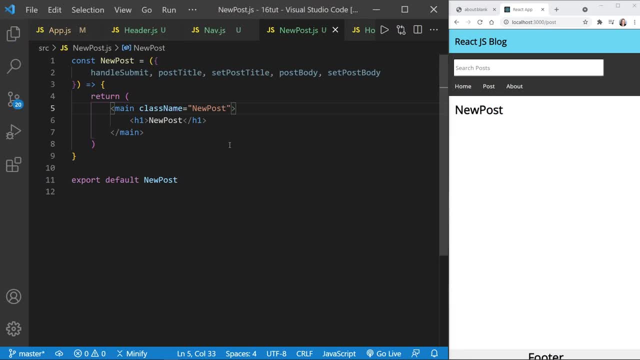 There we go. The main element has taken over With the formatting. Let's go ahead and change the new post h1 to an h2. And let's put a space between new post. But we'll leave that on the page. And the next element to add in the JSX is a form. 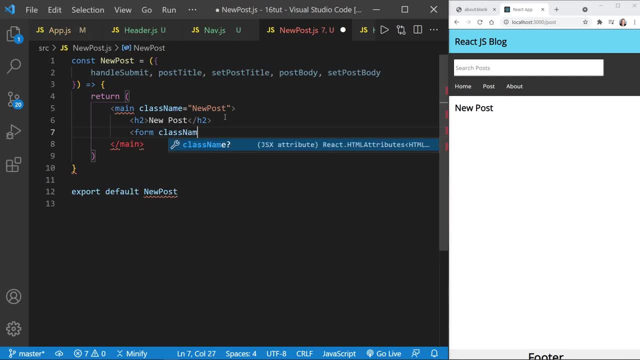 As we'll be submitting a new post And the class name here will be equal to new post form, And let's give this an on submit. But it might be different than you expect. Instead of a prevent default here, We're just going to reference handle submit. 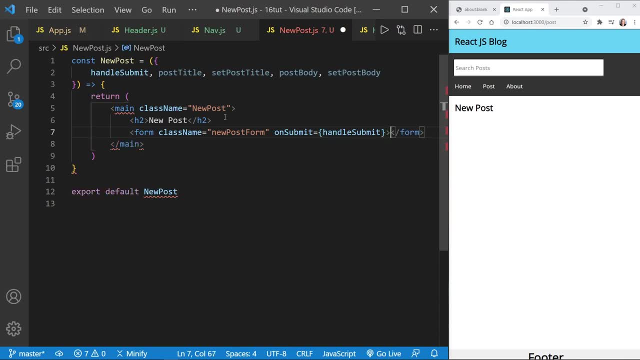 Now the interesting thing about this is it still receives the event. We don't have to have an anonymous function and specify e inside. If we just give a reference to a function like this, It will still receive the event And we can refer to that inside the function. 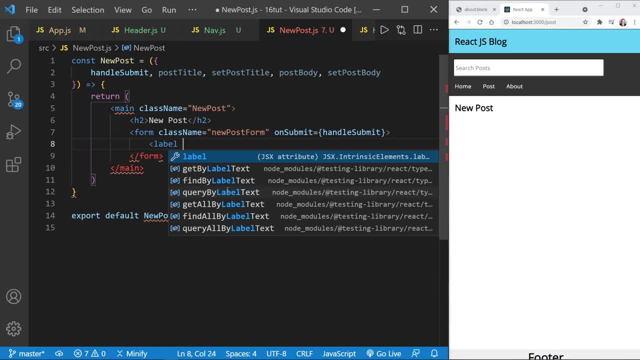 Okay, Let's put a label element for our input And this label. Of course, we'll have an HTML4 attribute And this will be for post title. Now, we're not going to hide this label either. We'll go ahead and show this on the page. 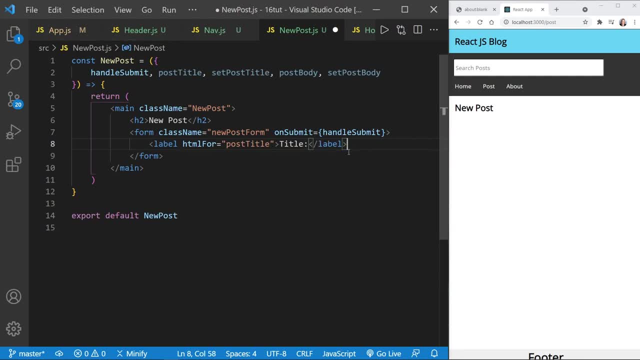 And here we'll have title, And now we can put our input for the title. And again, I'll put the attributes for this input in separate lines, So it will be equal to post title, As it needs to match the HTML4 attribute. 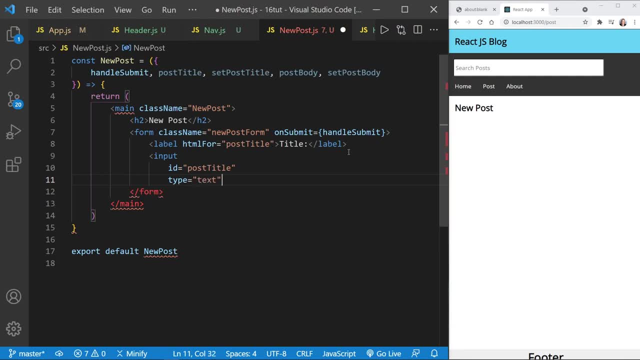 And the type is going to be text And we'll make this required, So the form will not submit without it, And this will be a controlled input. So we'll set the value equal to Post title And that means we also need an on change. 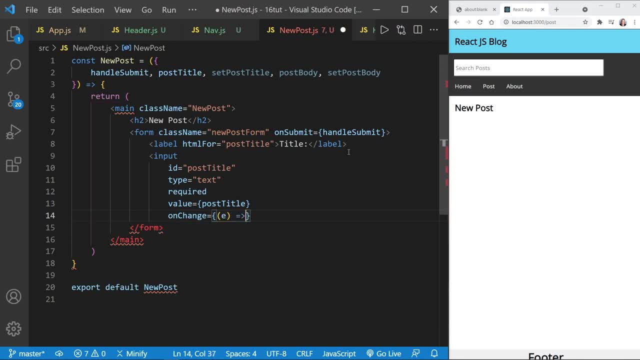 And we set the on change equal to That anonymous function. with the event We'll have set post title Equal to And we need a parentheses- E dot target Dot value. So this is a controlled input And that hooks it all up. 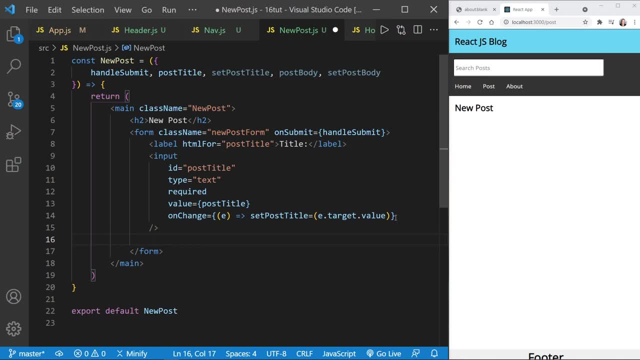 And we can close out that input. But we need the post body as well. So we need another label element With an HTML4. And this is going to be Post body And we'll just say post here For the label. 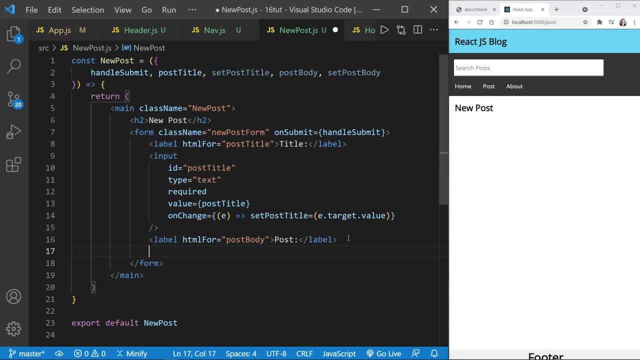 And now this won't just be an input, that's a text Or type text. We'll just go ahead and make this a little bit larger with a text area, And let's put the attributes for the text area on separate lines as well. 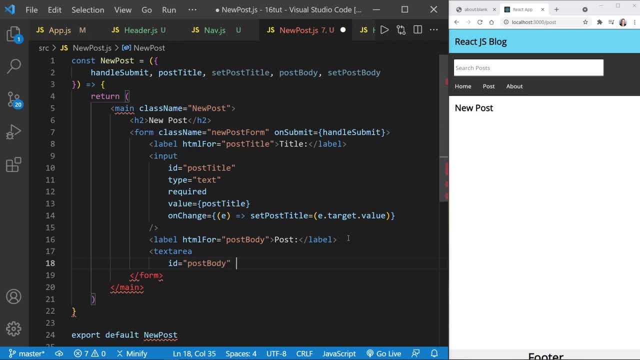 The ID will be post body. We don't need to set the type, as a text area is text. It doesn't have that attribute. We can make it required, And then let's make this a controlled input as well. So the value is going to be: 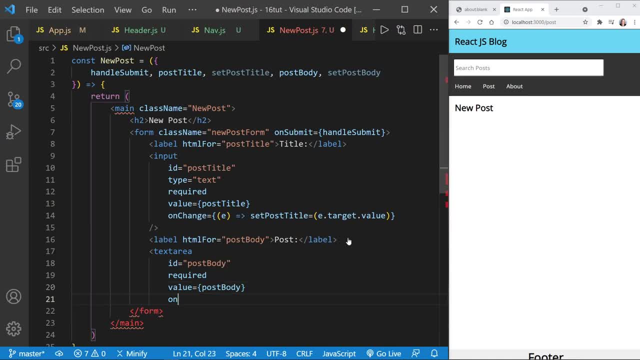 The post body that we received as a prop, And then we need to put an on change, Set that equal to, Once again, an anonymous function And inside the function we'll have set post body And have that be E, dot, target, Dot value. 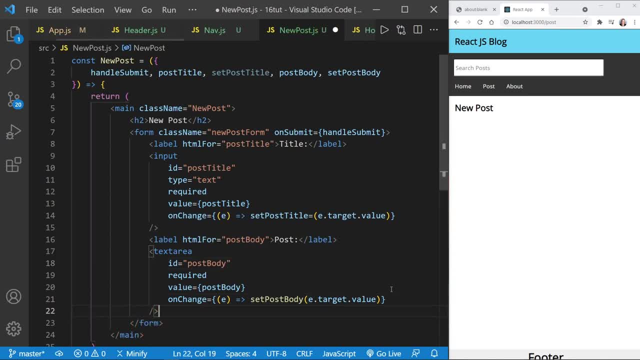 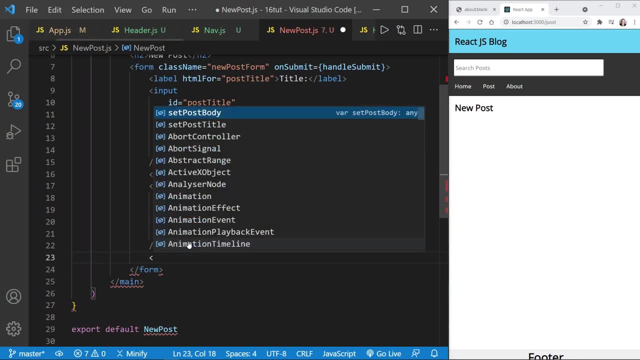 And now let's close out that input And we still need a button. So I'll scroll up just a little bit. And inside the form Let's put A button element And the type Will be a submit button And then on this we can just say: 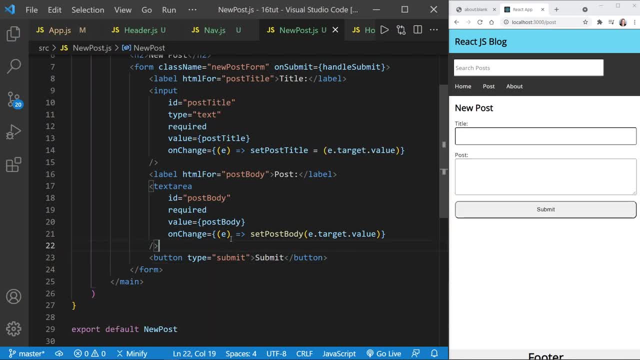 Submit, And that should finish out our form, And now we see everything over here in the page: We've got our title, We've got our post And we've got our submit button. We can't test this yet, though, Because we really haven't defined our handle. submit. 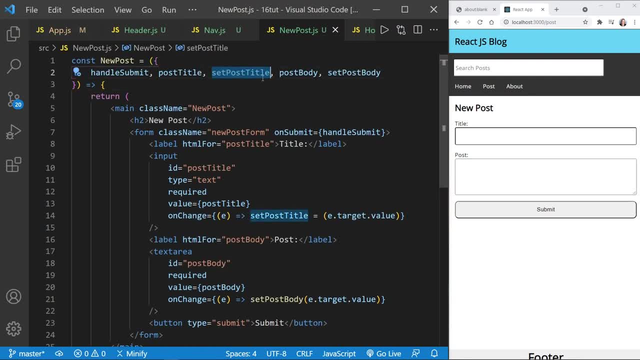 And it looks like I haven't defined the set post title. So I need to see what's going on with that And I see the problem. We've got an extra equal sign here. Let's eliminate that. And now we're using set post title, as it should be. 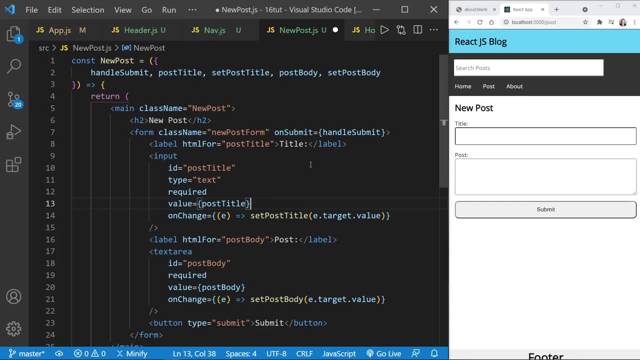 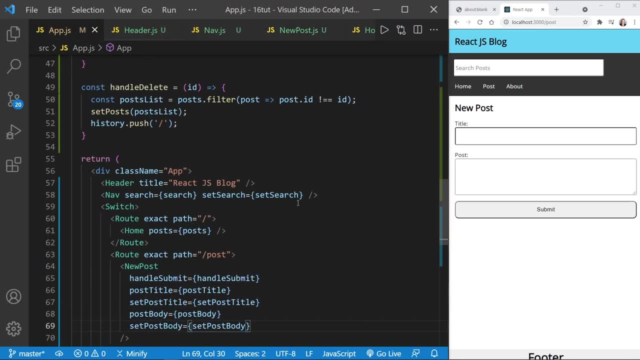 So if you followed along and had the same typo, I did Please change that. Everything looks good now. We'll save this And we need to go back to the appjs And define the handle submit function. As I've mentioned, The handle submit reference still receives the event. 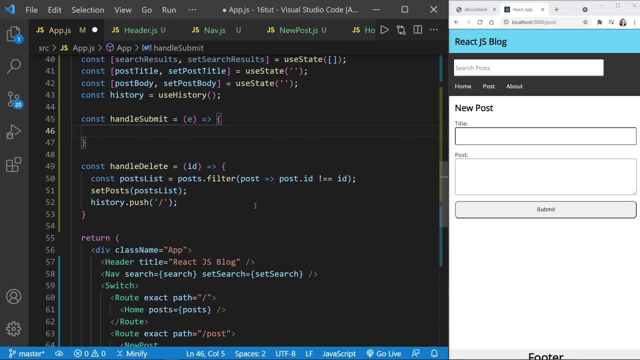 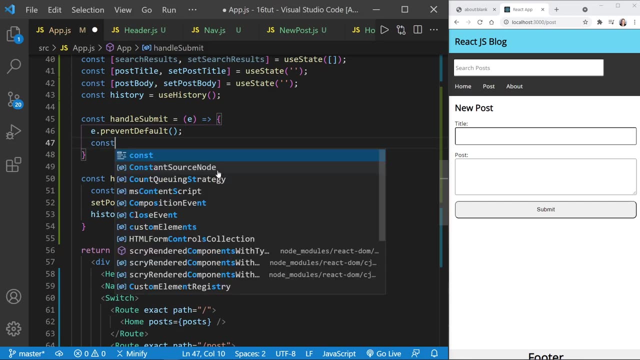 Even without the anonymous function specifying it back in the new post component. So here I just put the E for the event in the parameters And we'll reference that here And just call prevent default at the very beginning of the function. After that we need to define the ID for the new post. 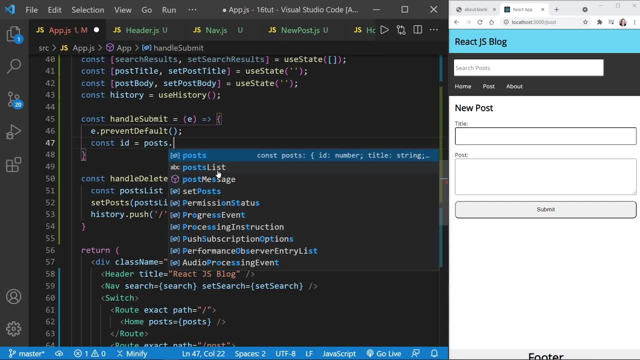 So let's set the ID equal to And let's check to see If the posts array has a length, And if it does, That means posts already exist, It's not empty. Then we need to get the last post And we do that with posts. 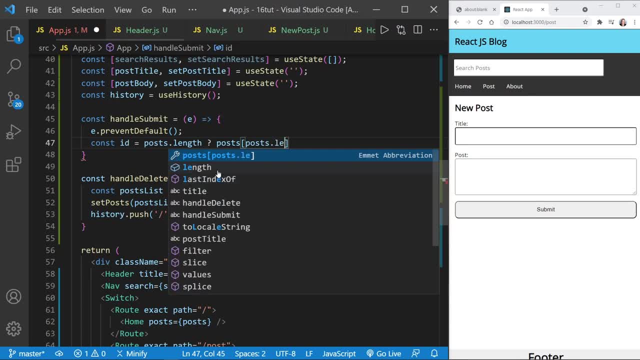 And now to reference the last post, We'll say posts dot length minus one, Because it should start counting at zero. So if you get the length, You've got the count of all the posts. You need to subtract one to actually get the last post. 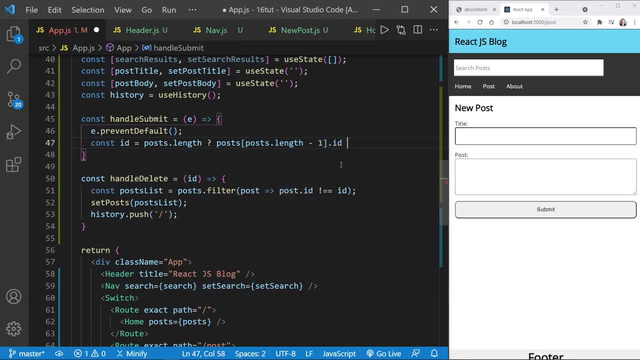 And after that we'll reference the ID property of that last post And then we'll add one to it. But if posts do not have length, That means the array is empty And we need to just give this post an ID of one. 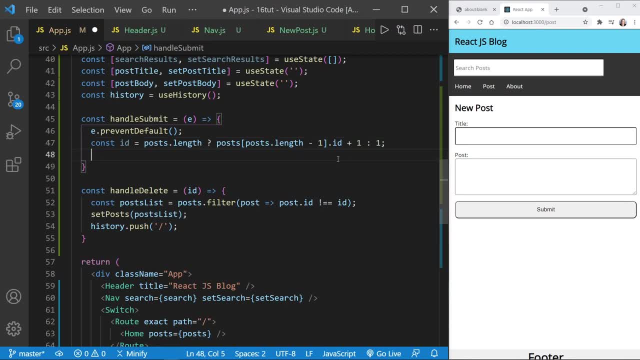 And now that we've defined the ID, We also need to define a date time value. I'm going to set that equal to an empty string for now. And now we need to import a dependency package that we haven't imported yet. I'm going to open a target. 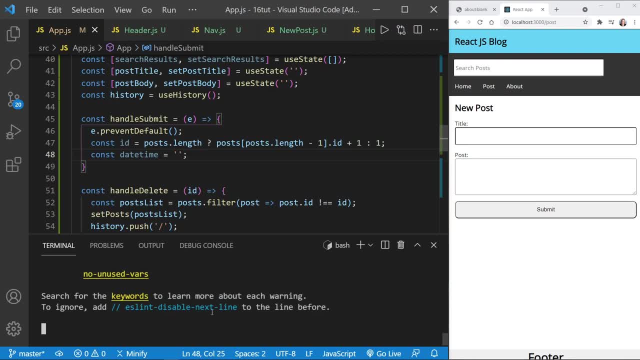 I'm going to go to the terminal window With control and the back tick And once I've done that, I need to go ahead and press control C To stop running our dev version of the React app right now. Now in the terminal window. 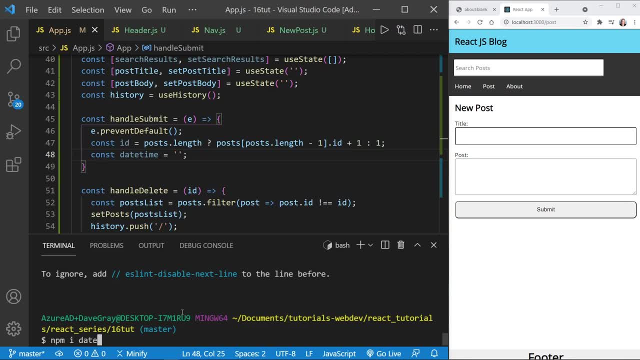 I'm going to type npm i And then date dash fns, Which stands for date functions, And then I'll type dash s. So we want to save this as a production dependency And go ahead and press enter And once it finishes installing. 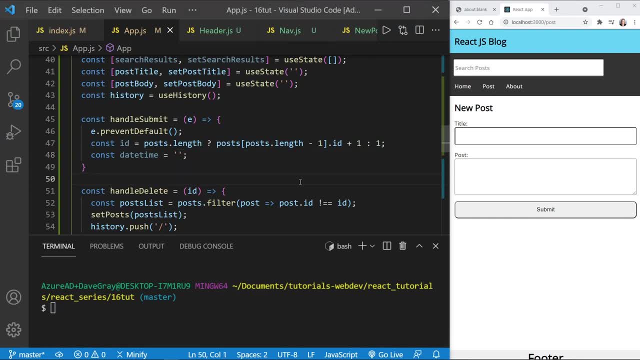 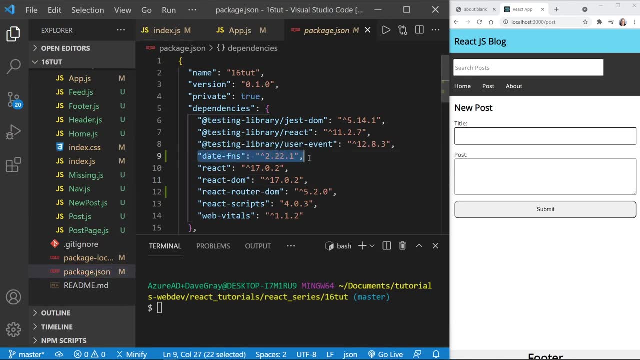 I'll come back. Our new dependency has finished installing. We can press control B to look at the file tree And check the package JSON to make sure it is there. And yes, Date dash fns is there. So I'll close the package JSON. 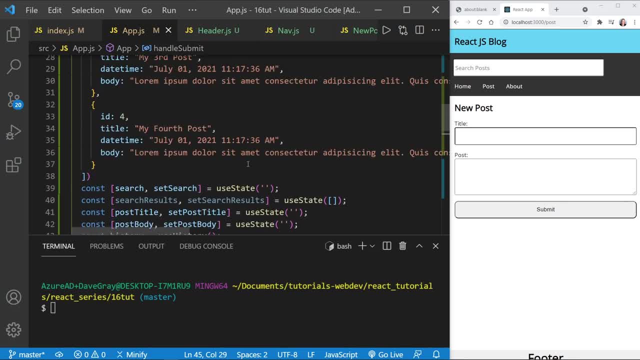 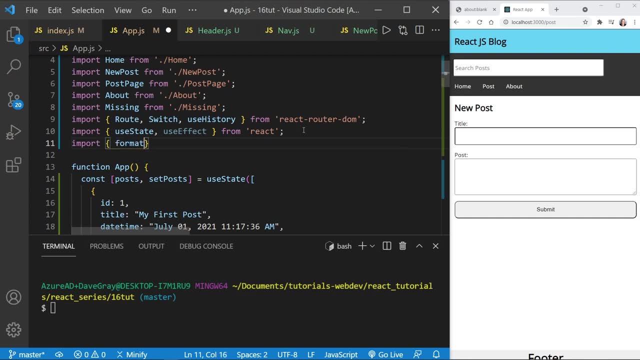 I'm going to hide the file tree again And at the top We need to go ahead and import this dependency as well. So we'll say import And we just want the format. So we'll destructure that From date dash fns. 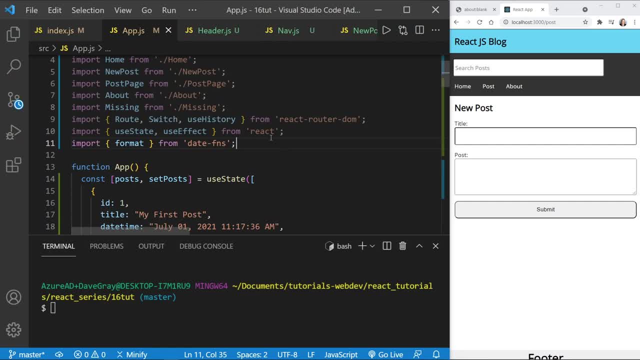 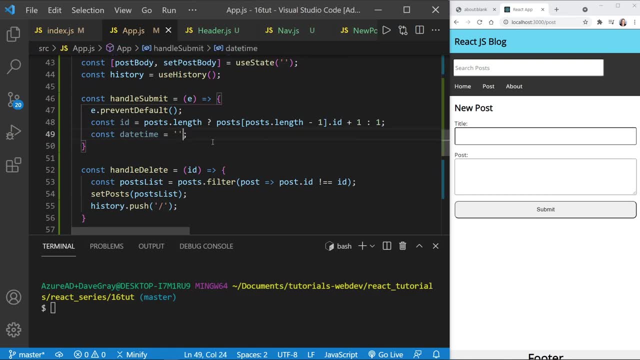 And save. And now I'll go ahead and come down here To the function we were working on, Handle submit, And we can apply the format in the date time. We'll go ahead and type format And then we need a new date object. 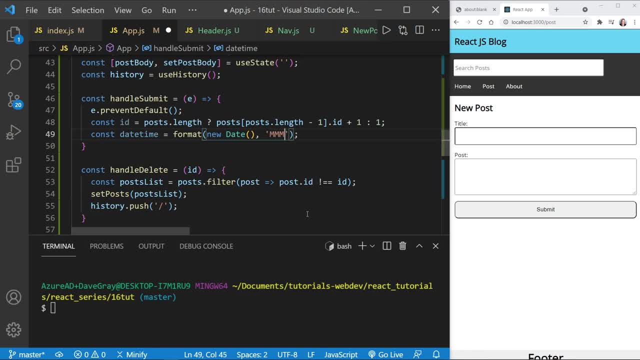 And then we can specify the format, And here I'm going to use four m's And then two lower case d's And then four lower case y's. So, as you might guess, we have month, date, year, And then we're using pp. 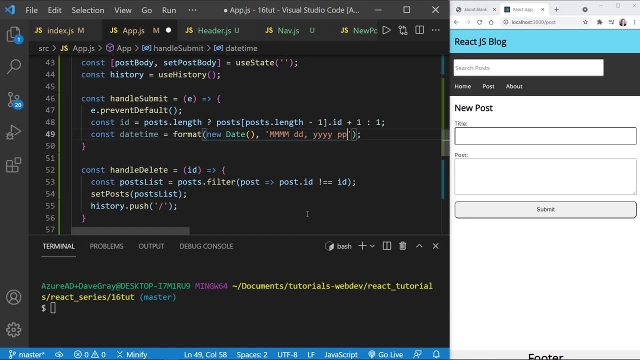 And this is going to specify a time. I'm not for sure why they use that format, But that's what it is. You can look up this package at npmjs as well, Or npmjsorg, I believe, To get the details on the date. dash fns package. 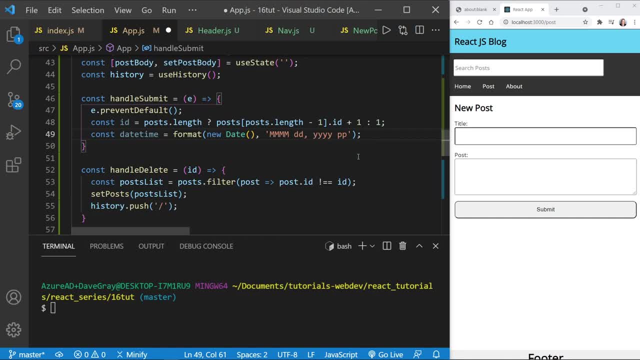 But this is what I pulled out for this project. Okay, Now that we have that And we're defining the date in the format that we want it, We need to create our new post. Remember, we are submitting a new post here And we're handling the submit. 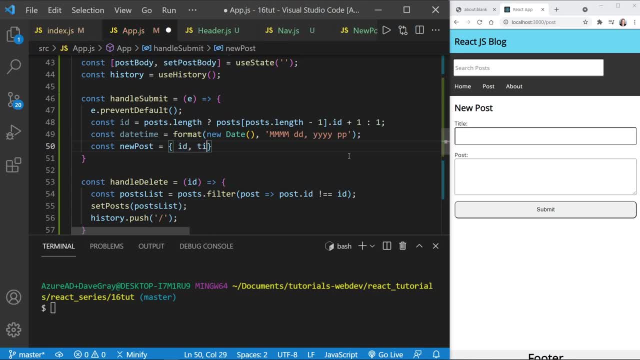 And the first thing we have in the post is the id, And then we'll specify the title, And that's going to be the post title- And then we can specify the date time that we've set, And then we'll specify the body. 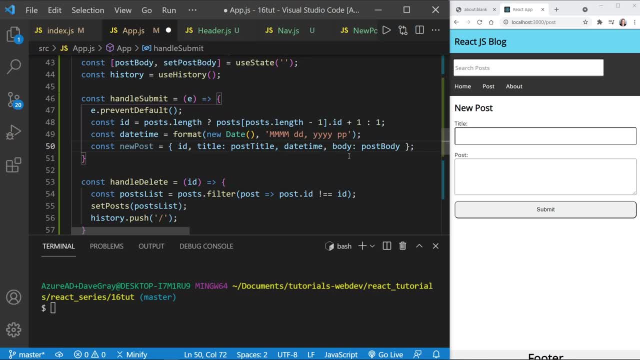 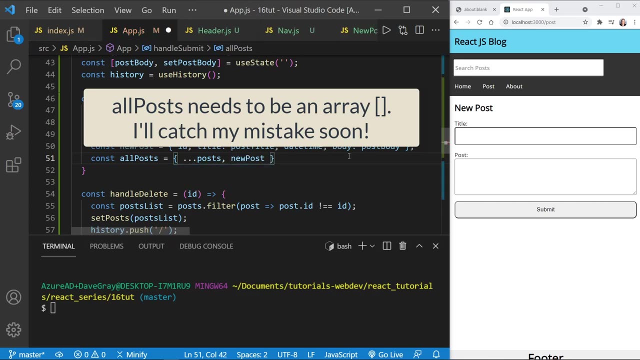 And, of course, that's going to be the post body And that is our new post. Now we need to create a new array with all posts, So we'll set this equal to the posts that are in state Plus the new post, And now that we have our all posts, 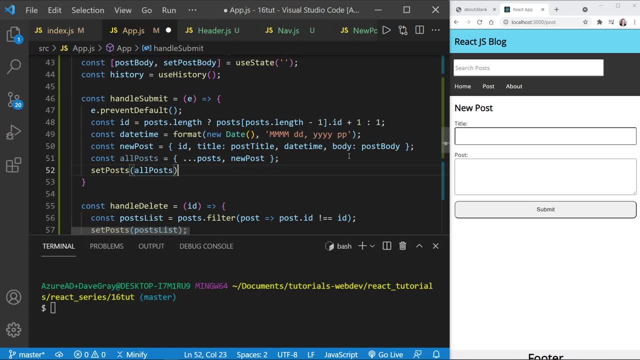 We can go ahead and set the posts as our new state And then we'll set the post title in the controlled input back to empty. So after we've submitted The new post, We won't have to delete what we've submitted to create another one. 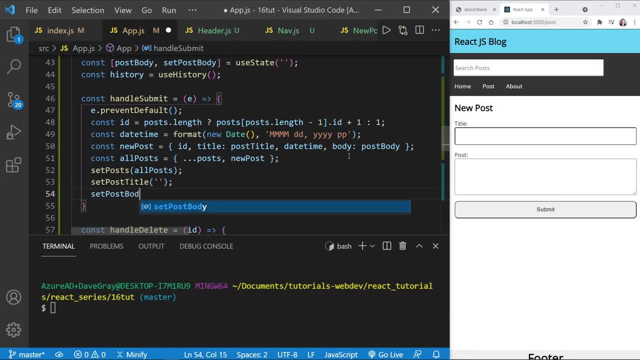 We'll just set that to empty. We'll do the same thing for post body. We'll set it back to an empty string And then, finally, We once again need to access the history and push, And let's go back to the home page. 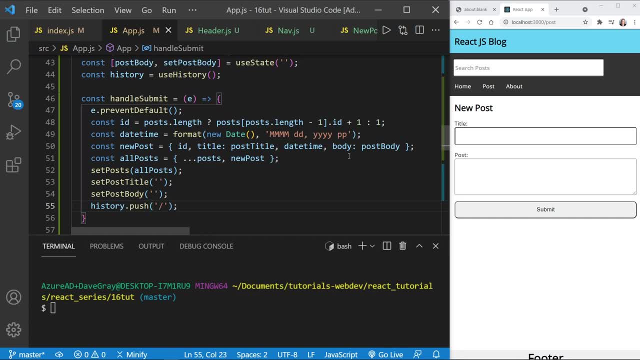 After we've created a new post, So we're not just setting on the new post page again. So now that we save all of that, We have stopped our dev environment with the react app To go ahead and install that date time dependency. 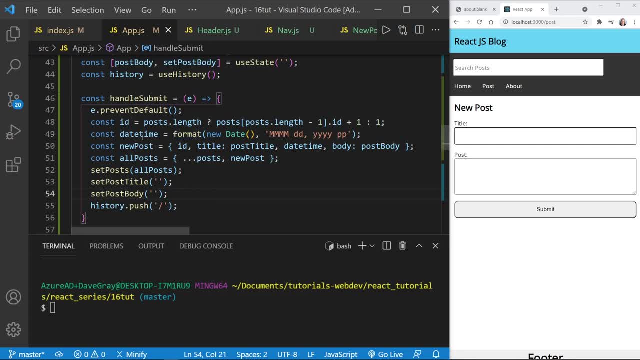 Where we pulled out format Or actually the date functions dependency That we're using for date time. So we need to once again start our react app With npm, start to try this out And our app is back up and running. Let's close out the extra tabs we have. 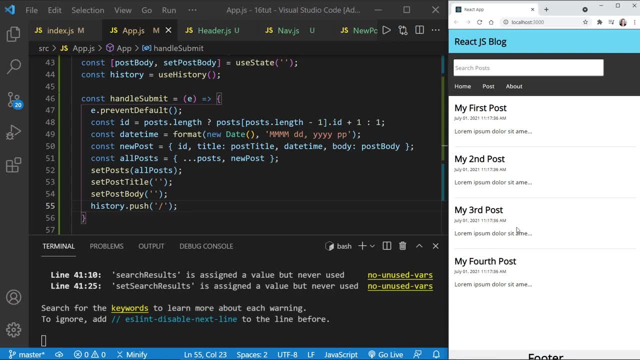 And this is the current one where our app is now running. Now notice, we got a warning here. Search results and set search results are assigned values But they're not yet used, So we need to go ahead and make the functionality For our search bar work. 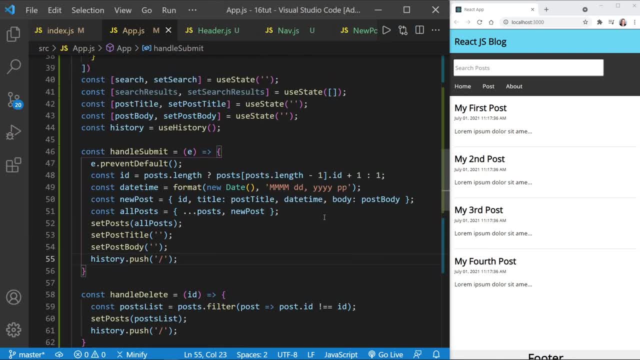 Let's close the terminal And we'll scroll up just a little bit here And we can see search results and set search results Have not been used yet. Right now they are using state And they're just assigned an empty array, So we need to change that. 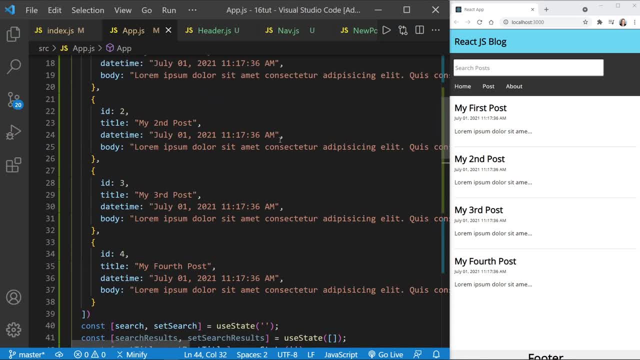 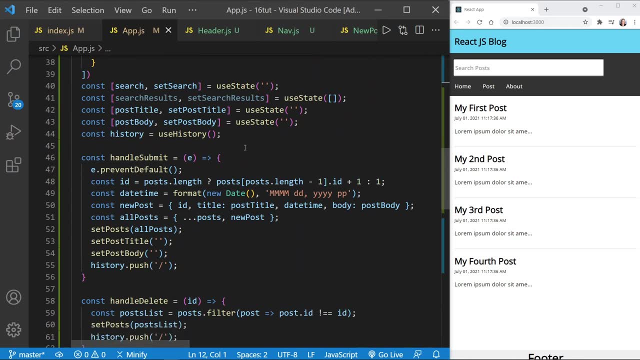 And we've already imported use effect. If we scroll up, I believe we'll see that There's all of our posts. But yes, we've already imported use effect, So let's go ahead and use effect now To work with this search bar and search results. 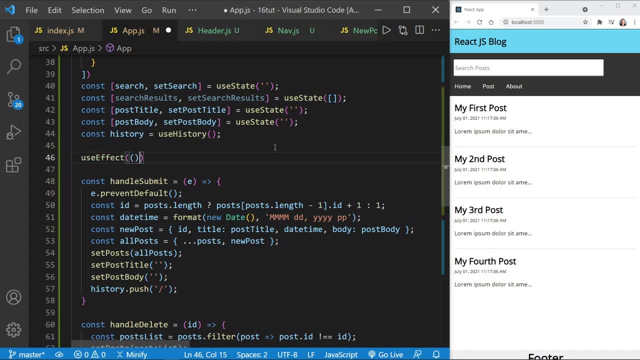 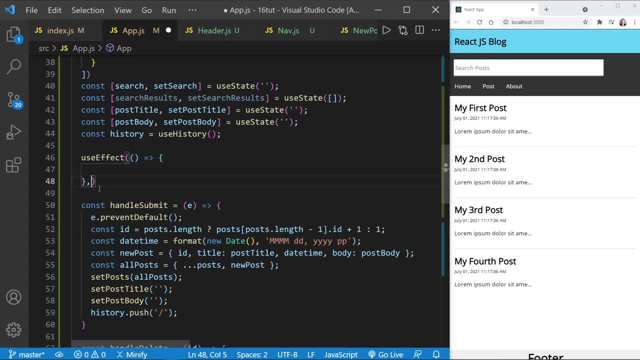 So we'll put use effect. Of course. use effect has an anonymous function, And then, after the function, we have to define dependencies for use effect, And when any of the dependencies changed is when use effect runs again. Well, we'll put that with posts. 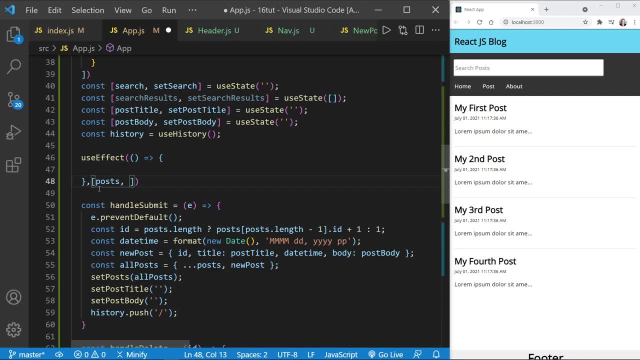 And we'll also set that to work with search, And so now, as our search input provides new data, We could go ahead and provide new data here for the searches. We can essentially filter the posts that we have down to what matches our search. 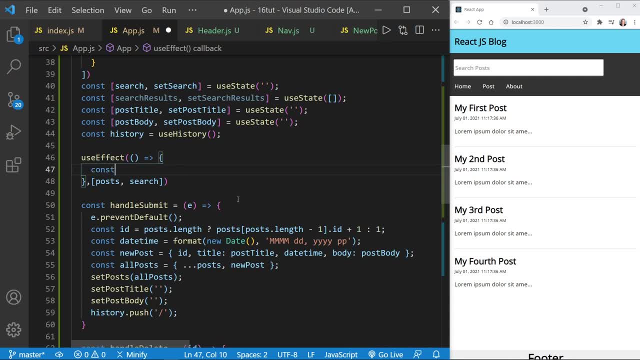 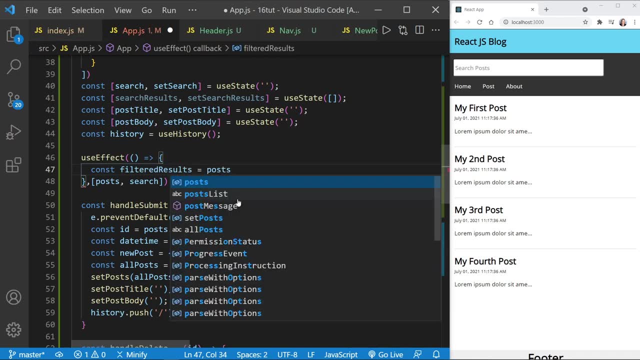 And so that's why those are both dependencies. We're going to define something here called filtered results, And we'll set this equal to the posts dot filter, And now we can just say for each post: And inside of that, Inside of this, we'll need our parentheses. 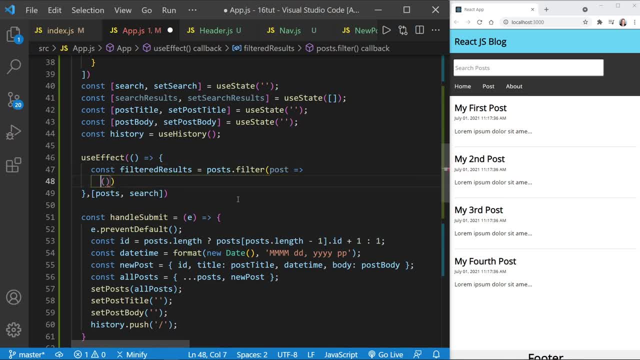 And let's go ahead and put this on a separate line, Just so we can see everything. And now we'll have inside the parentheses Another set of parentheses to specify the post body. And we need that because then we're going to add a dot to lower case. 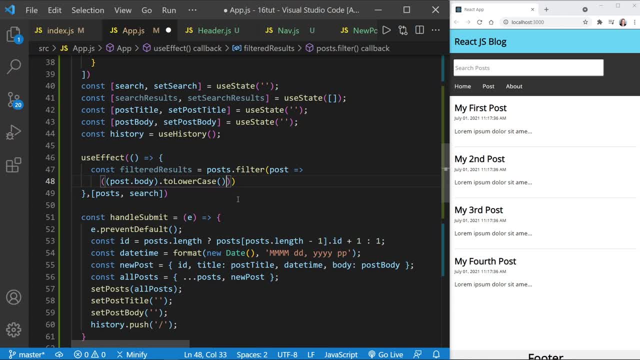 And this will set everything in the post body to lower case And now we've got the outer parentheses And then we can put dot includes. So we're checking to see if the post body includes, And by setting everything to lower case We're not being specific about whether it's capitalized or not. 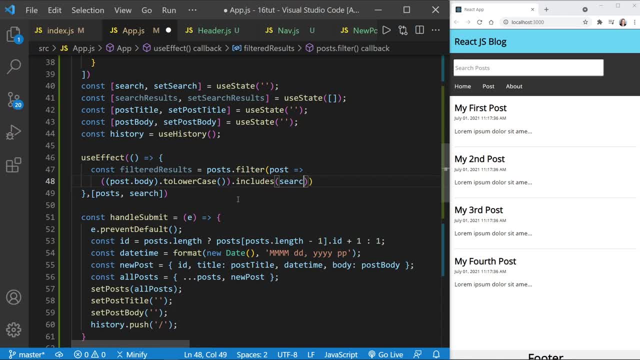 Our search will work either way, And then we can use our search value And also set it to lower case So it could possibly match. And there we've got our full filter for the post body. So we set the post body to lower case. 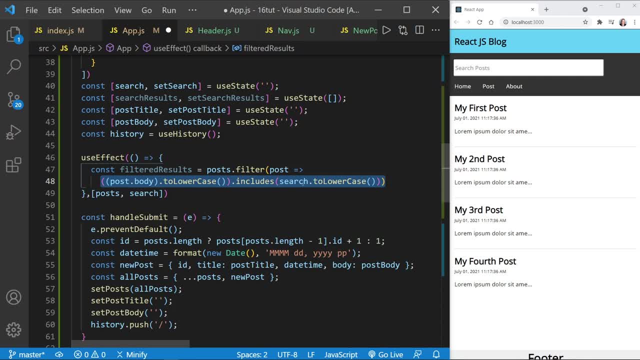 We also set the search to lower case And we're checking to see if the body includes What we're searching for Now. after that, This, of course, This yellow one here, Or gold, if you will- Highlights our entire filter function. 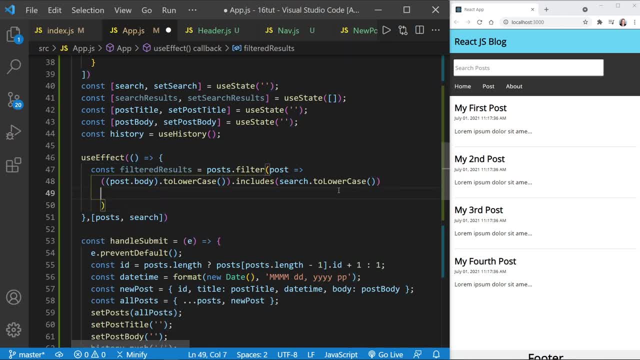 So I could put this on a separate line Or even underneath. After that, we need to use an OR, Which is also considered a short circuit operator, But this is OR And we want to do the same thing, But not just for the post body. 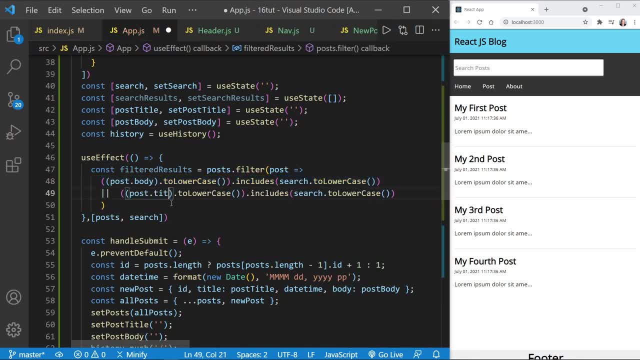 We also want to do it for The post Title. So if either one has what we're looking for, This is what we'll search for And contain in the filtered results. So now I'll put that closing one back there at the end. 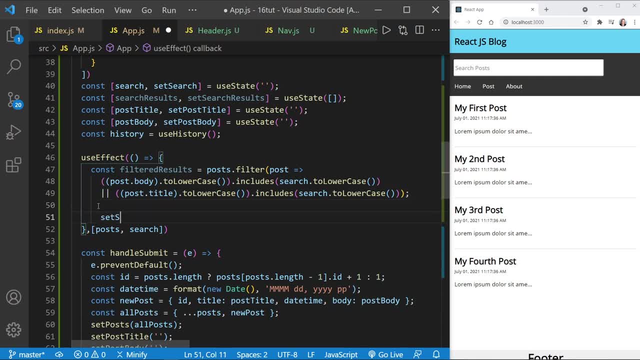 And we've defined our filtered results. After that, let's set the search results, But instead of just setting them equal to the filtered results, Which we do need to put in here, Let's think about our posts Right now. the oldest post is always at the top. 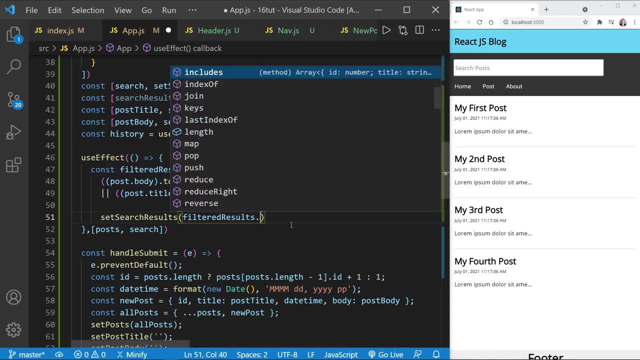 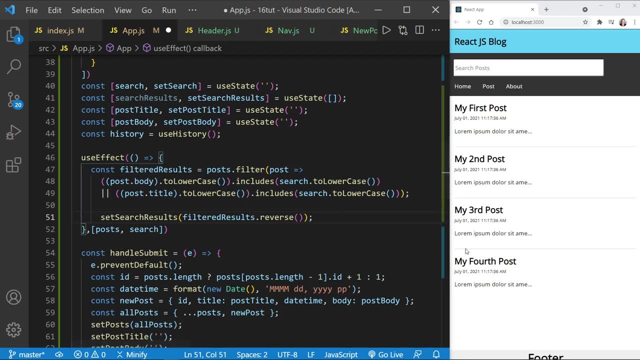 We'd rather see the newest post, So let's go ahead and set this to reverse, So our search results are reversed Now. this still won't change this right now, Until we change what we're sending to our home component, So we save that. 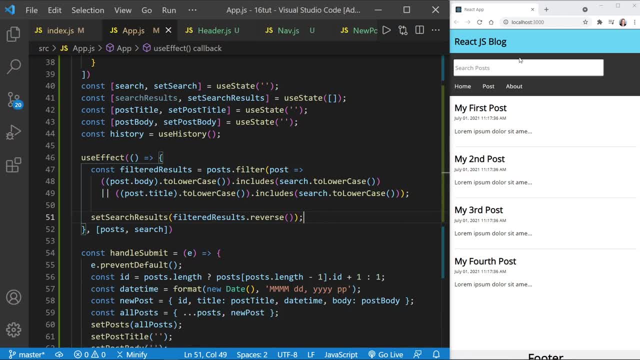 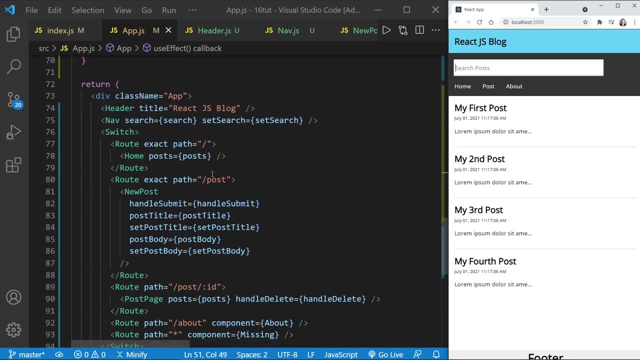 And we have the search results, But we don't see anything happening. yet If I type in F or FIRST, Nothing is happening here with the feed, And that is because our home component below Is receiving the posts and not the search results. 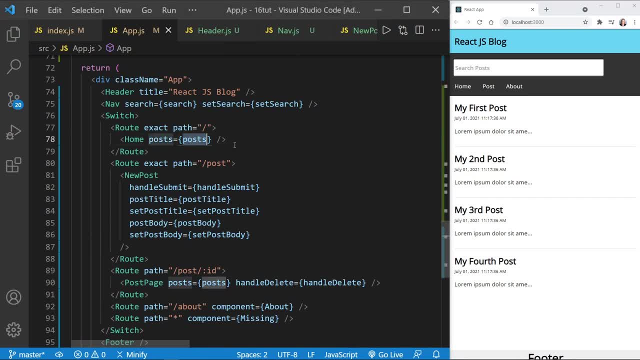 So let's change that. Let's still refer to it as post, As we do throughout the child components, But here we'll pass in the search results And now let's save this, And quickly we see it is now showing the fourth post at the top. 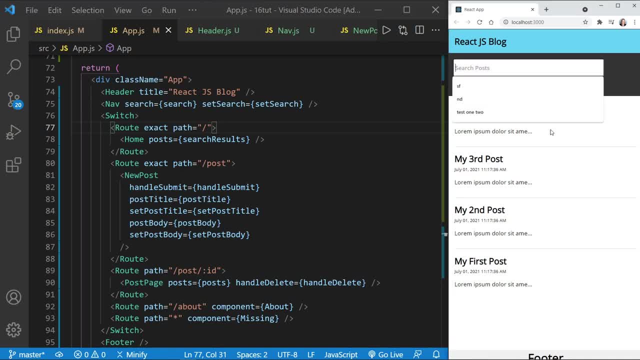 Instead of the first. It's got the reverse order And now we should be able to search posts, So I'll type 3 for third, And yes, that works. 2 for second, F for first and fourth, And they both show. 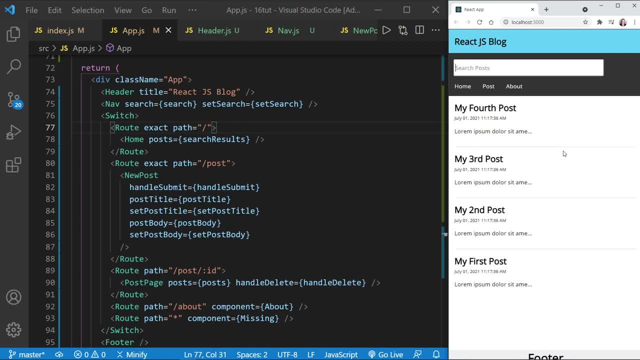 But if I put an I it's just the first post. Now they all have the same body right now, So let's see if we can add a new post. Call this test post And we'll make a short one And we'll add that. 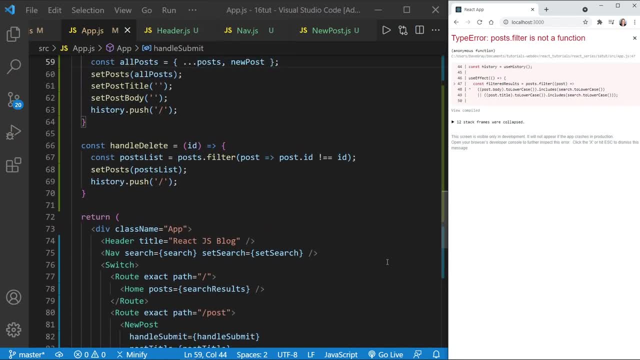 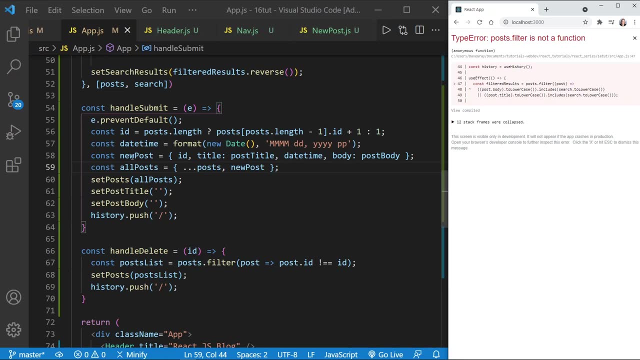 And we've got an error. Let's see what's wrong with our handle submit function, Because we were trying to submit a new post And I think I see the problem. We created a new post object And then I was in the mode of creating objects. 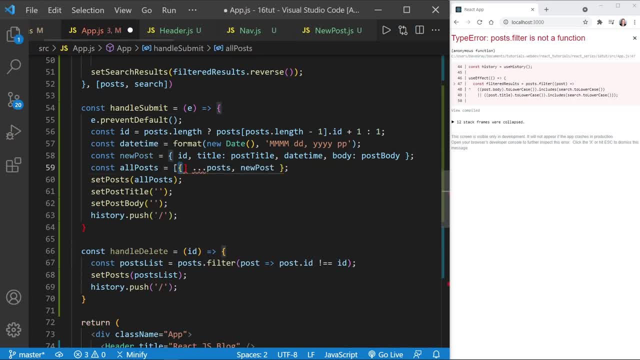 But our posts need to be inside of an array, So if you followed along with that problem that I created, Please fix it. And this should be an array. There we go, And let's change this other curly brace to a bracket also. 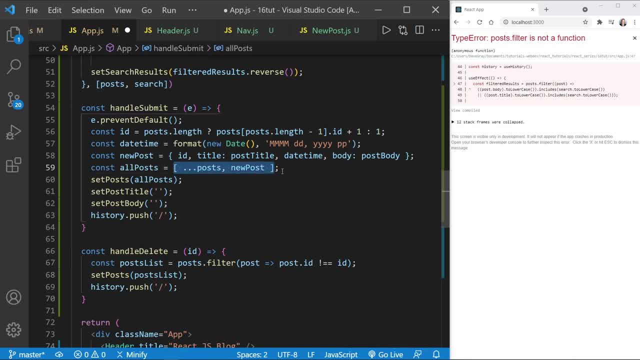 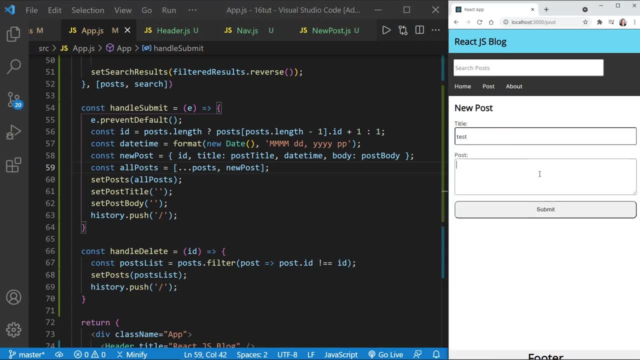 Now we have a new all posts array And that should be what we expect. Let's save And let's try to create this new post again. So we'll just say test And inside of here we'll just say yay, Because we want a short post. 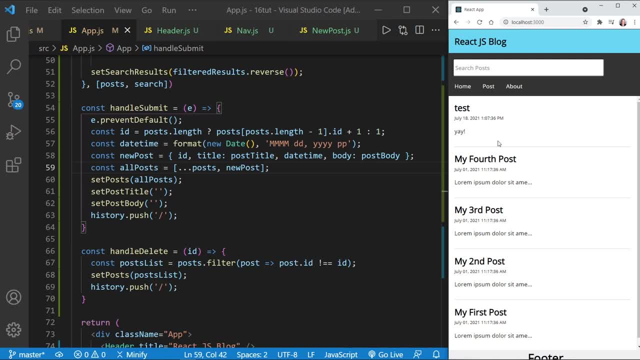 And now we've got our new post, And the new post shows up at top And it's less than 25 characters long. So this goes back to where we set the ellipsis if it was 25 characters, And then we put an ellipsis after it. 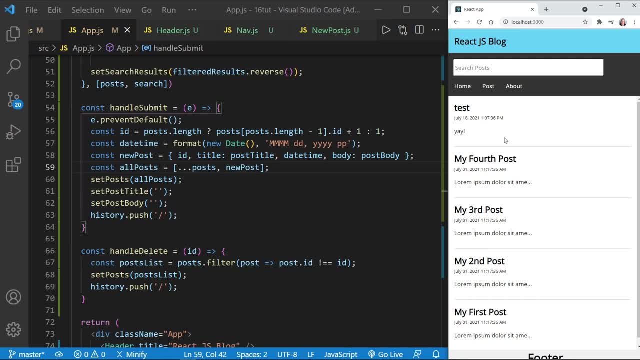 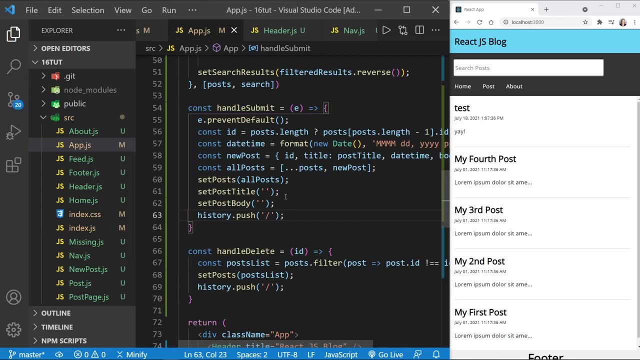 But if it's not, we just show the full post, And that's what we're doing here, with no ellipsis. So everything works as expected. Now I'm going to show the file tree again. We've really only got three more components to complete before we're finished. 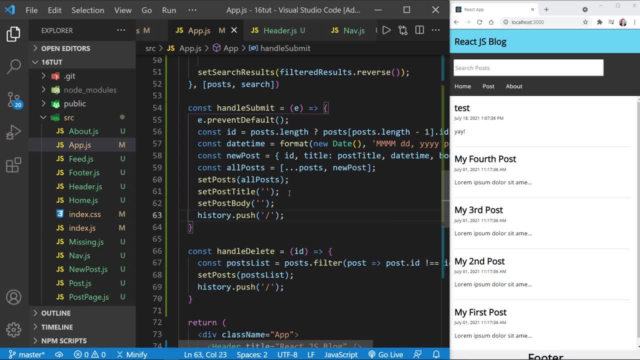 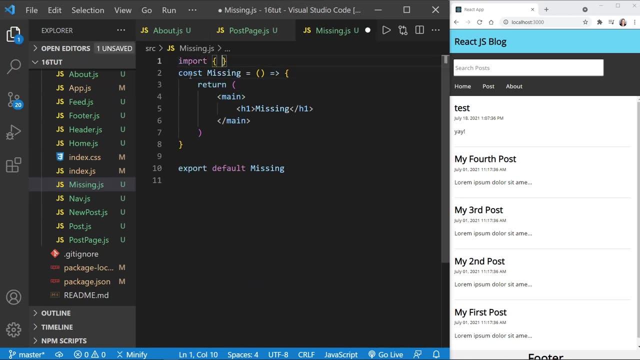 And that is the about component, The missing component And the footer component. They don't really receive props, So we should be able to do this fairly quickly. I'm going to go to the missing component, first Missingjs, And at the top of missing we need to import from react-router the link again. 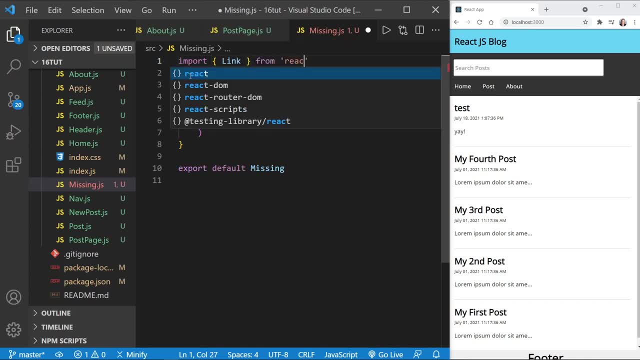 So we can link back to the home page And we'll say from react-router-dom, And after that I'm just going to highlight the main element here inside the JSX And paste in what I have And you see a class name of missing on the main element. 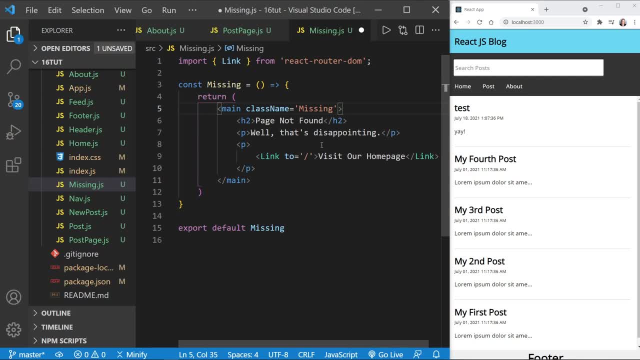 We get an H2 page not found instead of post not found that we had for our post page when a post was not found, And then we link back to the home page. So let's save that, And we should be able to test this by just putting anything after our URL there. 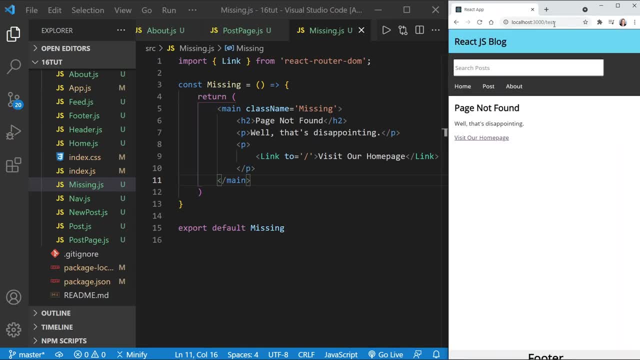 So let's just put test And we don't have a test route And it should bring up our missing And it does. Page not found. Visit our home page- An interesting thing to note. Let me go ahead and delete the third post. 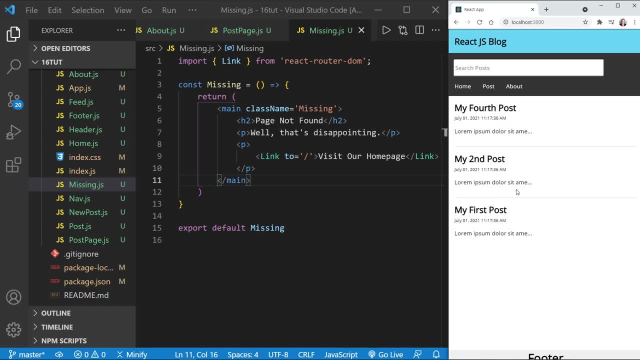 Now we've deleted those And again they load statically when the app reloads. If we go to a missing page, like we did there for test, now the app essentially reloads, Because after we've routed to the missing, if I go back, the third post is there again. 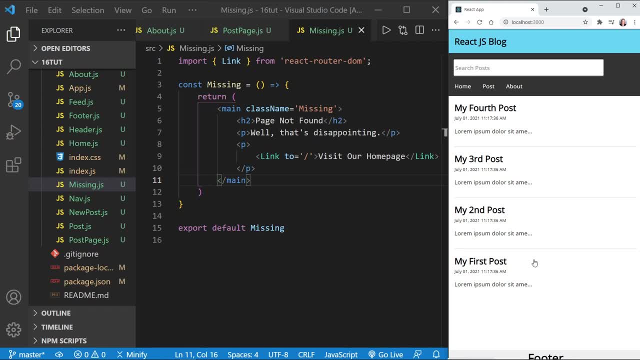 So that's worth noting, that the app essentially reloads. Now, of course, you wouldn't be using static post, Using static posts with a production app, But that's what we're doing here in development And that's why the third post may come back. 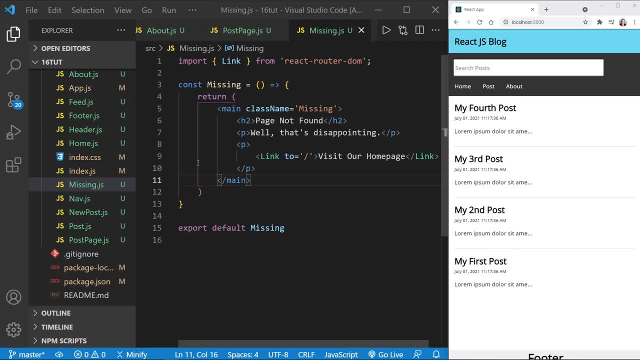 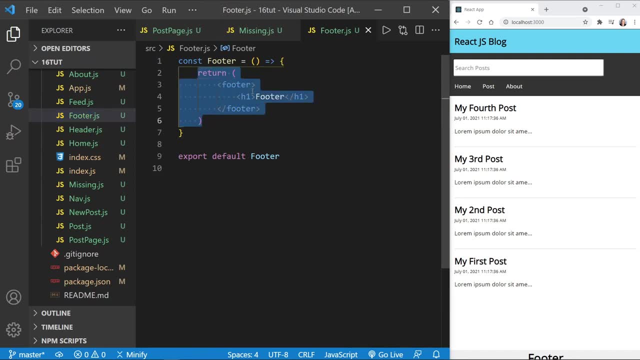 Or any post you've deleted after you go to the missing page. Now let's go to the footerjs, And inside the footerjs there isn't anything to receive as a prop. again, I'm going to select everything, including the return, And just paste in what I have. 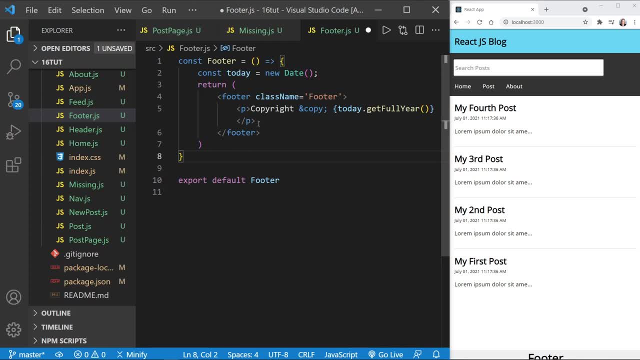 And here I'll press Alt Z to wrap just a little bit So you can see anything that might be missing. But you can see, I'm just defining today As a new date before the return in the component And then I'm referencing that with the copyright. 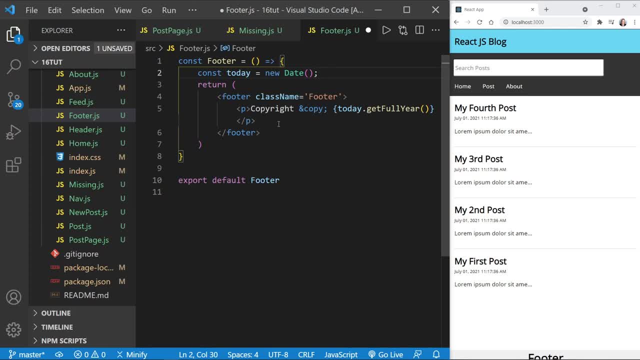 And I say today: dot get full year, So I get the current year, And now let's save this. And our footer should change. And yes it does. It's a little bit hidden down here And I'm not sure why, But here we can see the full footer right now, if I expand the page. 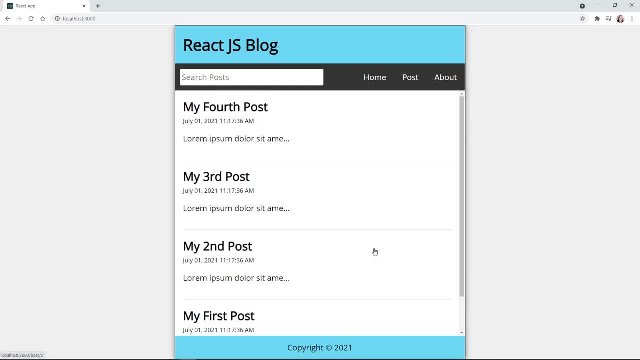 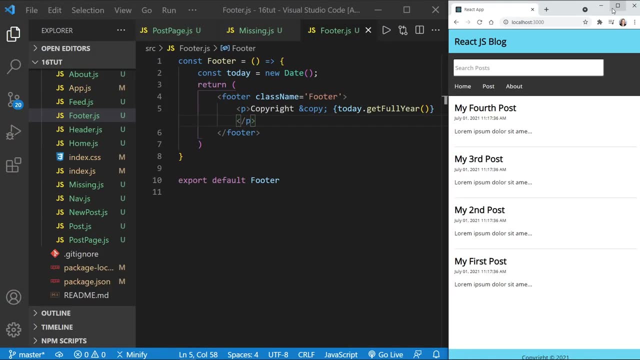 And we see everything, And it's static as well, So we can scroll the main area of the feed, And the footer is still visible there. Now I'll resize- And for some reason it's just scrolled off here- just a little bit. 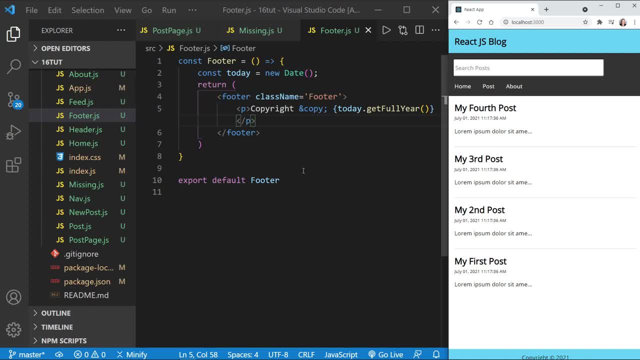 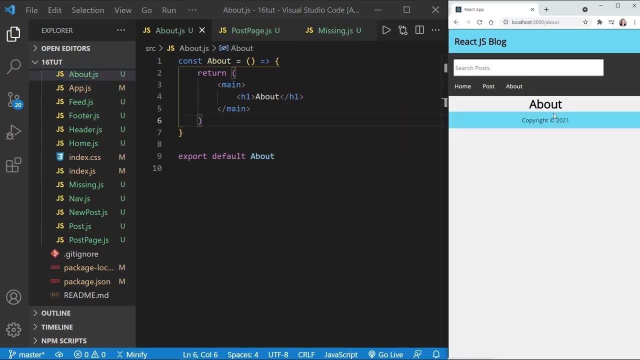 But it wasn't doing that for me previously. Okay, So there, we've got the footer And now we need to go to the aboutjs And I can click the about link over here And we can see we still haven't added anything for about yet. 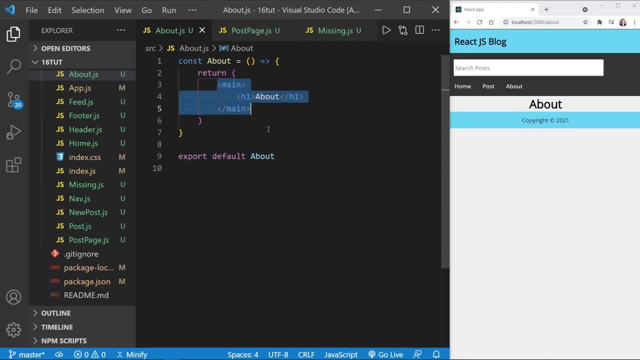 What I'm going to do is just highlight the main element and everything And paste in what I have- Alt Z again so you can see the full thing. And again, we changed the about to an H2.. We added the class name about. 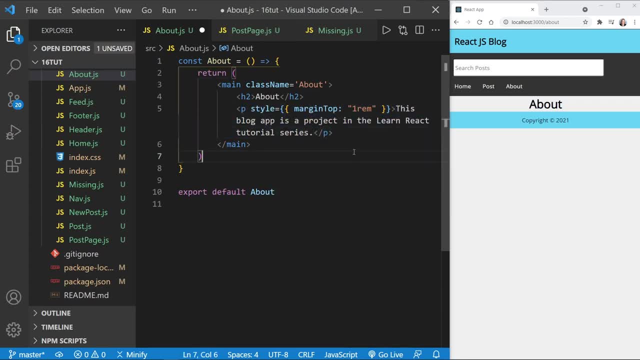 And then we just put in a small statement about what the project is, And we'll save that. And now our about page is what we expect it to be And it fills out the space. So, about works, We have our new post page. 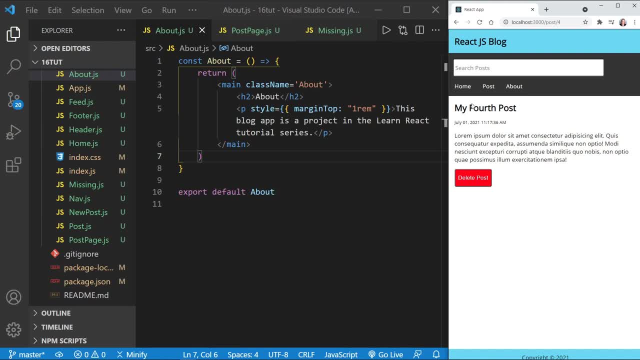 We have our feed. We can go to the details of any specific post in our feed And everything is working as we expect it to, And this is a great start to this project. In the future, we're still going to add additional features to this application.